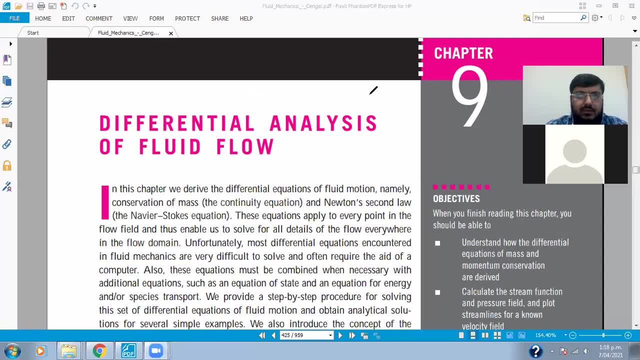 So we are going to understand all the two points. But if you don't move the screen, how do you know the difference. On today's lecture, let's talk about differential analysis. Because your problem is the first point The fourth point Oh yeah, but when the experience보다 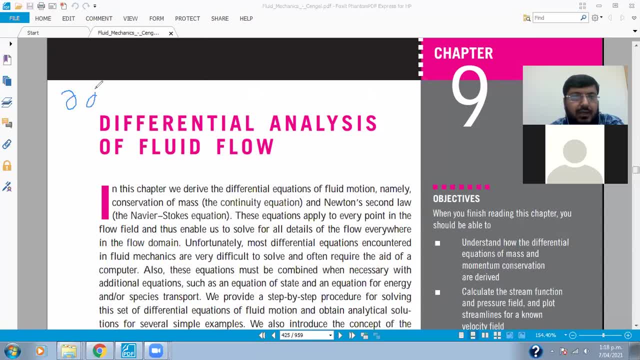 karen differential analysis. Differential means that we are talking about an infinitesimally 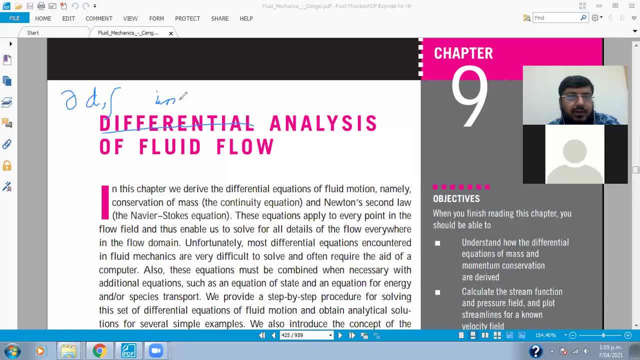 small particle. Infinitesimally small particle. Differential analysis of fluid flow. Differential analysis means that we are talking about an infinitesimally small particle. Infinitesimally small particle. Infinitesimally small particle. When we develop its mathematical model then it will come in the form of these three. In the form of partial, differential and integration. 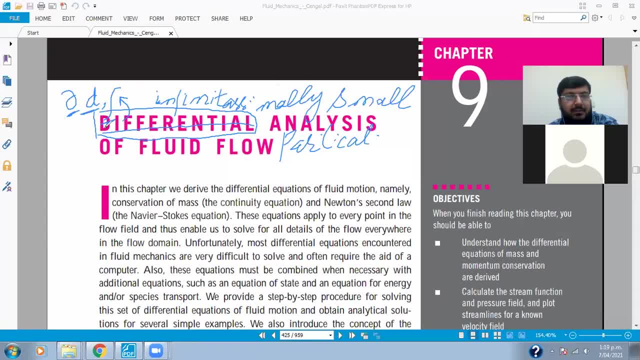 When I will talk about it then the story of fluid mechanics started like this. There is the core above it. D Narghagrava düš worked in the fields as a statistic teacher. At that time we跑 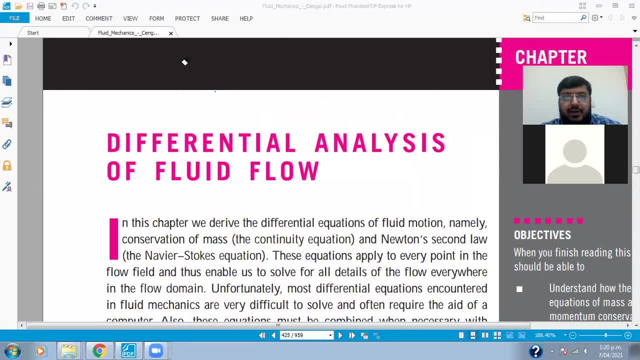 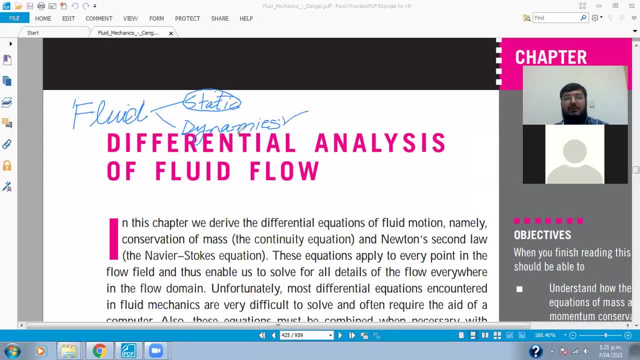 so it means , Now let's say what we are stuck with. Because that's what we are doing what we are called a Warriors, So what we are called a Warriors, is in dynamic condition, it means that your fluid is in motion form, you can't say that we have taken water in a glass, this is also a fluid mechanics, if you simply say that you have taken your water in a glass, then this is also a fluid mechanics, but when we talk about fluid, sorry I am saying mechanics, then this is also a fluid problem that if you have taken water in a glass, but when you talk that the fluid is moving from one 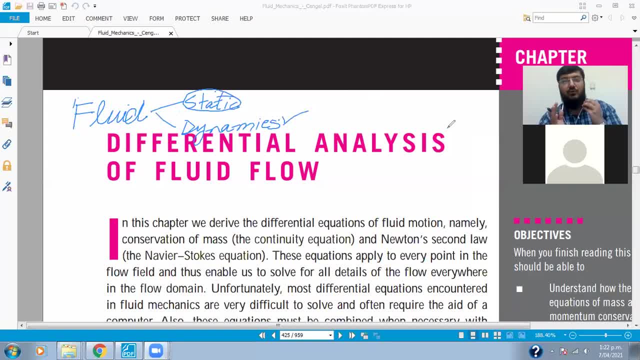 place to another, then you are talking about fluid dynamics, now when we have such a problem, okay, now I am going to tell you the story of fluid mechanics 2, okay, when we have such a problem that when we move the fluid from one place to another, now when we move that moving fluid in terms of mathematics, 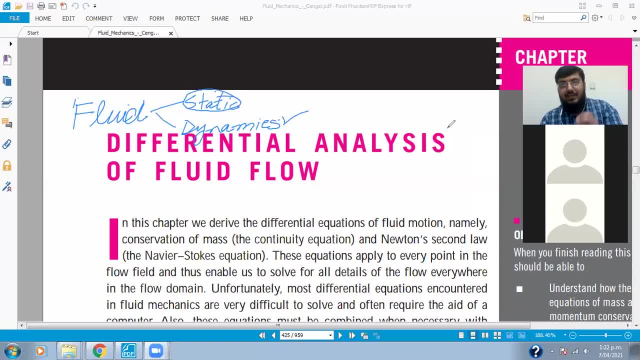 we have to write in terms of mathematics, as I told you, what is mathematical modeling, mathematical modeling, fluid mechanics, in chapter number one, he has made three figures, in which he tells that we first have a physical situation, then we write its governing equation, then we take its solution, so fluid mechanics, if you see this in chapter number one, then you will get that book, 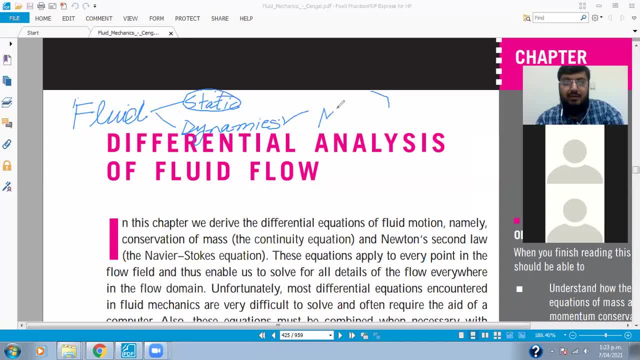 then we can get that article and what is that article, mathematical modeling, 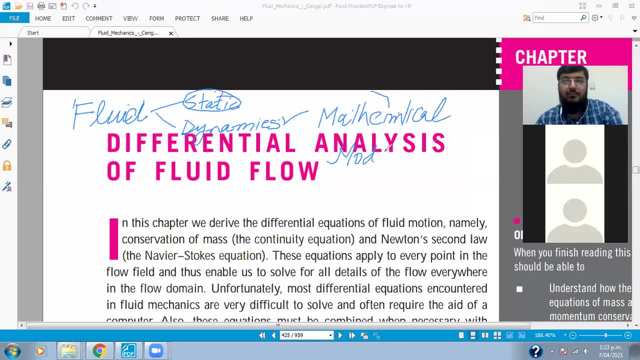 it is okay, you will get this technique, then mathematical modeling is that you have a physical situation, you have to write that in terms of mathematics, okay, so that you can take a solution deal for it, for exampleI will talk about, That is example, let's say, as I said, if a person wants to solve a mathematical problem, for example that person knows that a particular thing, then he will be happy to take the solution, If this person wants to solve then that system will be able to solve it very easily. need to build and resolve a disease pain After y in order to succeed In來說тов 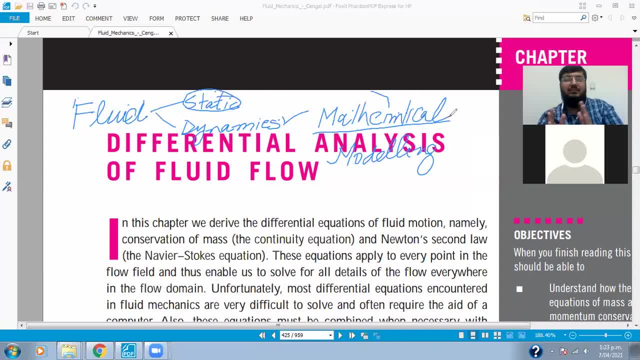 If I say that I have a car, it is going from one place to another place. I say, tell me this. How will you tell me? You will tell me that there is a car which is moving from one place to another place within this specified period of time. So I will say, son, this is a lot of words. So you simplify it a little bit and tell me what this is. 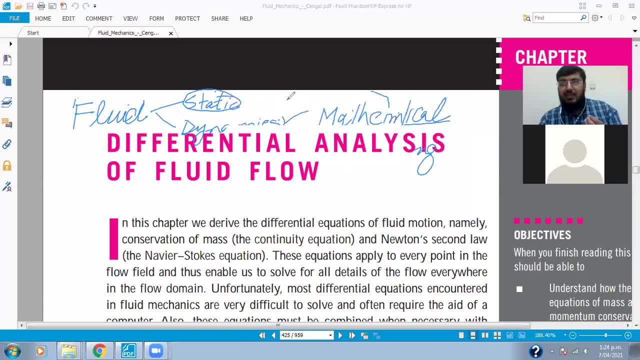 Okay, in the language of mathematics. 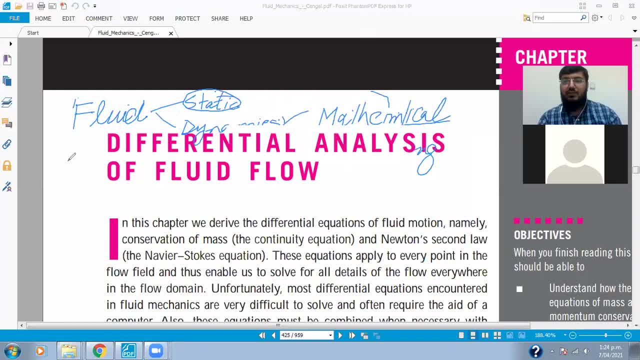 So what will you say? You will say that the mathematician is so long statement that the car is moving from one place to another place within this specified period of time. 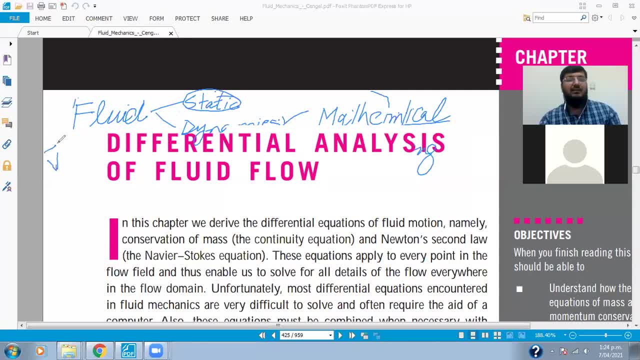 What will he do? He will do like this, he will put V vector and he will say simple DX. 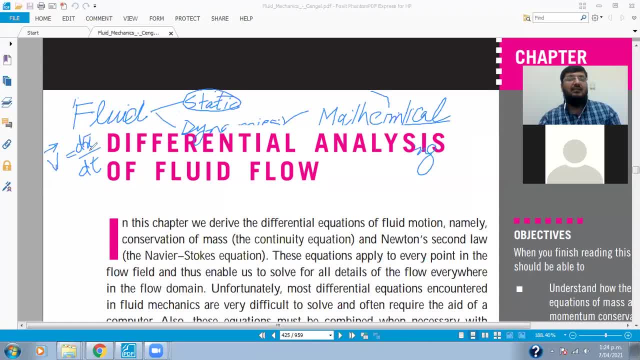 By DT, he will say that the X is a displacement, so we got a small mathematical model, we got a small mathematical model, now if a mathematician will define this thing, he will just say that DX by DT, after doing that, it will go, which is as easy as me, it is simple, he will simplify it further, he will put a dot on V. So the person who knows the mathematical language, what will he do? He will read it out. He will read it out. 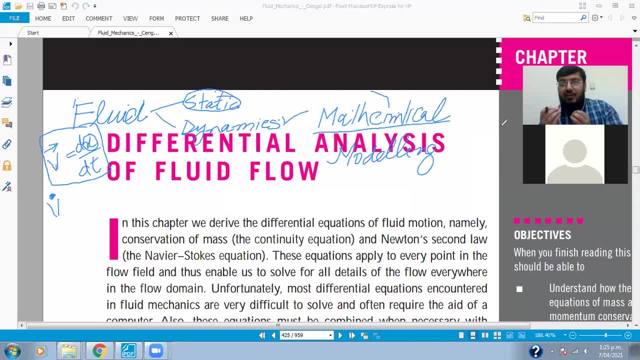 After reading it out, he will simply say that what does V dot mean? V dot means the rate of change of displacement. Now you have read it, right? 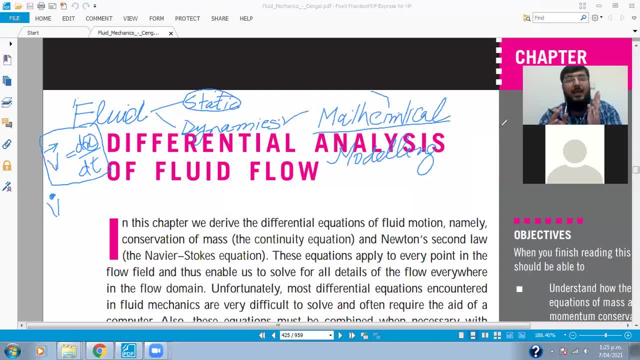 So now we have taken the physical situation and written it in the mathematical model. Now when we have to calculate the velocity of something, then we have to find the velocity of some car, so we put DV by DT. 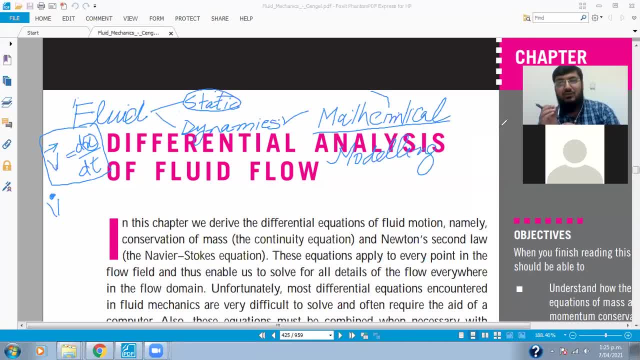 And we will find out the velocity of that car. Okay, this was for solid particles. Okay, this was for mathematical modelling. I am repeating all of these things, son. 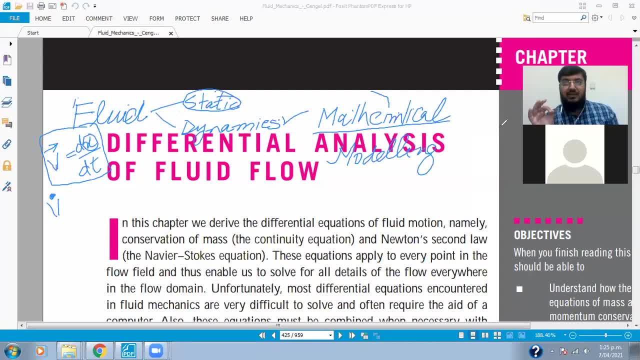 That first of all, when we talk about fluid dynamics 2, then we will talk about fluid mechanics. Oh sorry, fluid dynamics. In mechanics, static also comes. So we will talk about fluid dynamics. Okay. Okay. 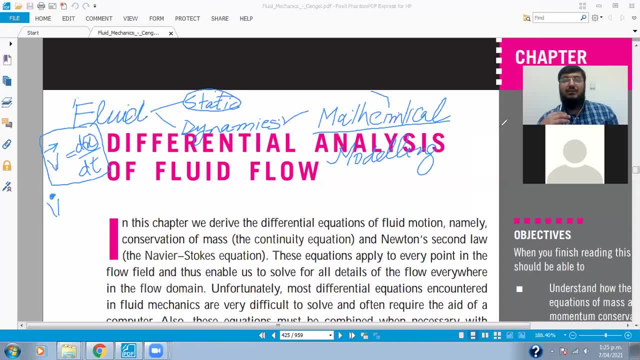 When we talk about fluid dynamics, then in our mind, we have to keep in mind. question is that if there is a flow in a channel, then you tell me that if I have to measure the properties of the fluid, I will say that water is flowing in a canal, you measure its velocity and show me its pressure. So you will say that sir we have two methods to calculate it. We have two methods to calculate it. Number one, I will experimentally throw a sensor in it or I will put an experimental device in it so that I can know its velocity and pressure. This will be done in one way. What is the second way? The second way is that I have two methods. 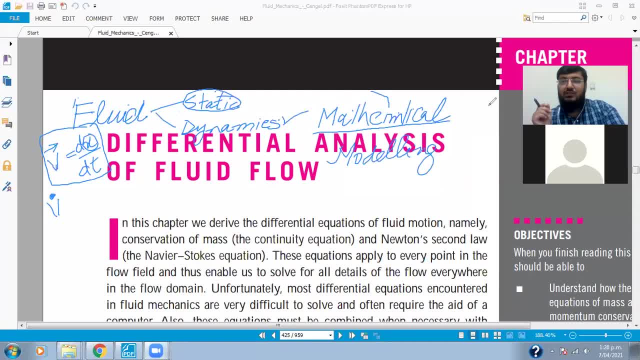 If I have some mathematical relations in which I put values and that mathematical relation will give me the value of that thing. For example, usually I say that if I want to find a rectangle area, then there are two ways. Either you take a scale. After taking the scale, you find its area. Or the second thing is that you just measure its length, measure its width. You have the initial conditions, you plug the length and width in the formula. area is equal to length into width so you have its area did you get it? so these mathematical models, mathematical equations what they are doing is that you theoretically on the page you are on the page 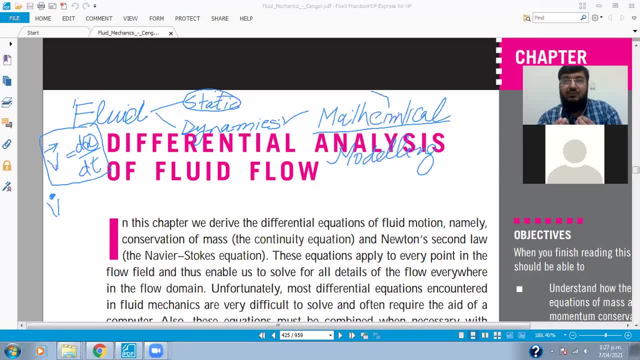 you are giving the solution for example 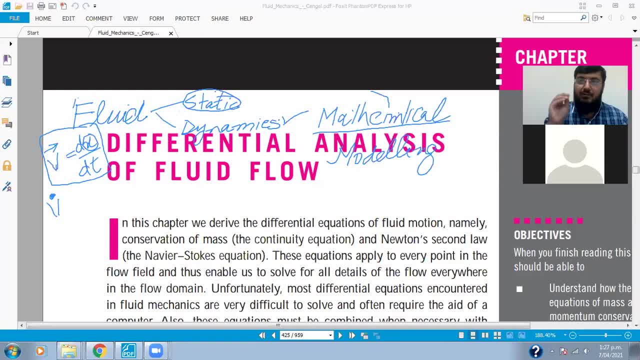 I gave the example of area you just plugged that thing in the formula of area you got that thing 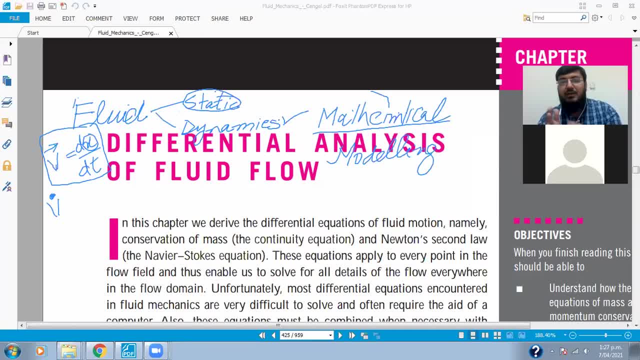 similarly when we talk about velocity we don't have to give such a long statement that the car is moving from one place to another 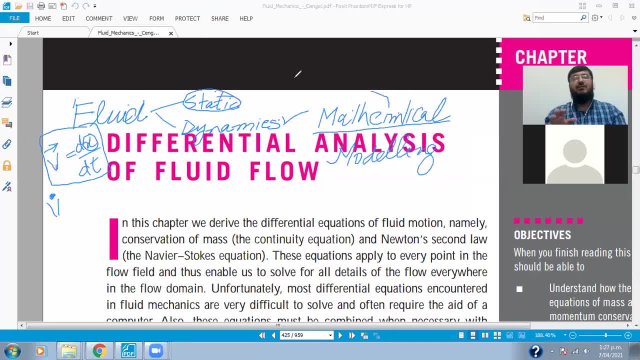 we are just talking we say this and find out that it is dx by dt 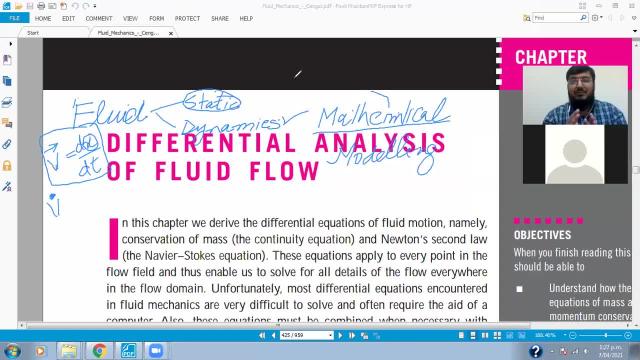 so these are the mathematical models mathematical model means that you have to pick up the physical situation 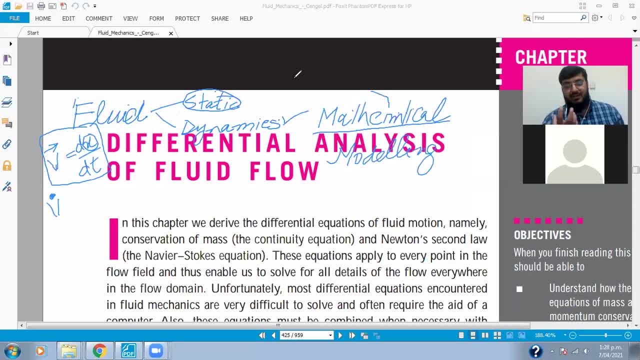 and bring it in terms of mathematics 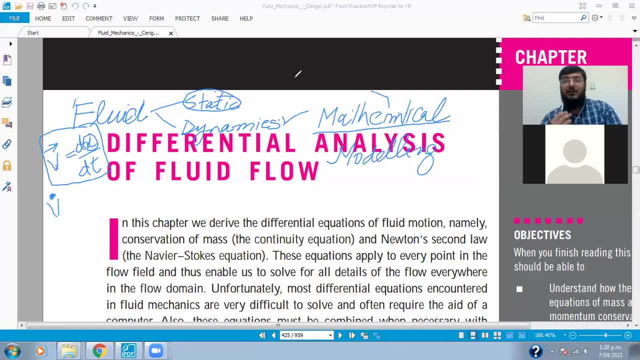 now the question is that the continuous models that you have continuous processes 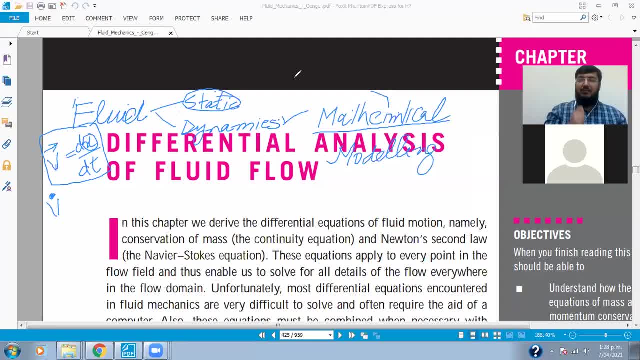 like I say that I have taken a hammer I have hit the hammer 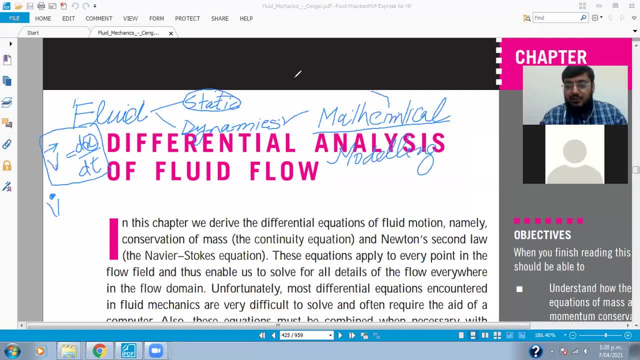 I have hit it and stopped it so this is not a continuous process this is an individual process that I have hit one step and finished it but what about flows 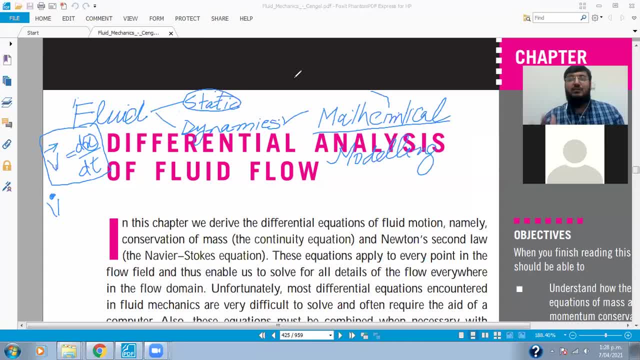 if one thing is going from one place to another then it is going continuous it is going continuous so this means that when we talk about flows of flows so this means we would talk about continuous 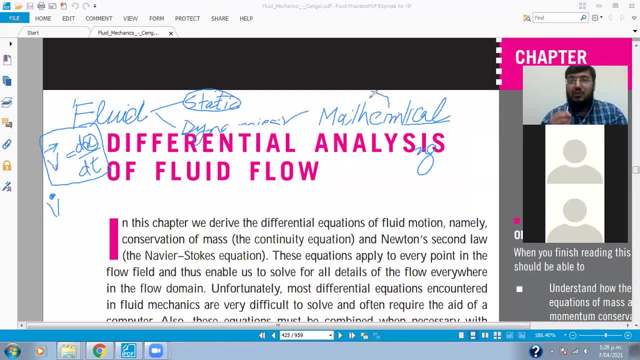 so if we talk about continuous flow then the mathematical model of that the mathematical model of that how will it be it will be in the form of partial 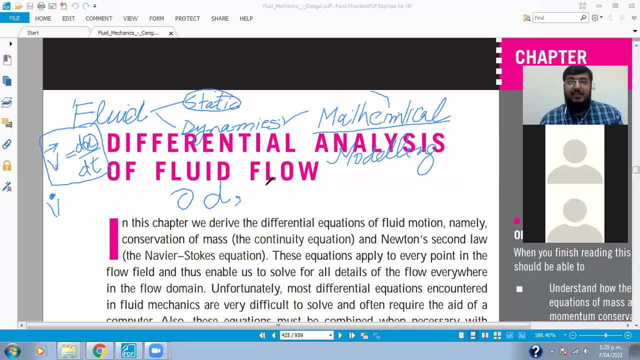 or derivative or in the form of integral whatever the fluid the fluid flow 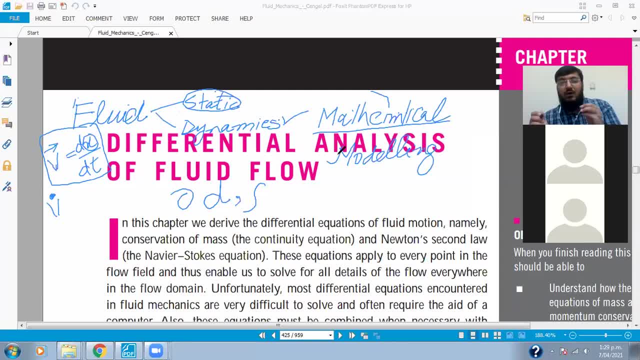 will go from one place to another the model of that will be finalized in that 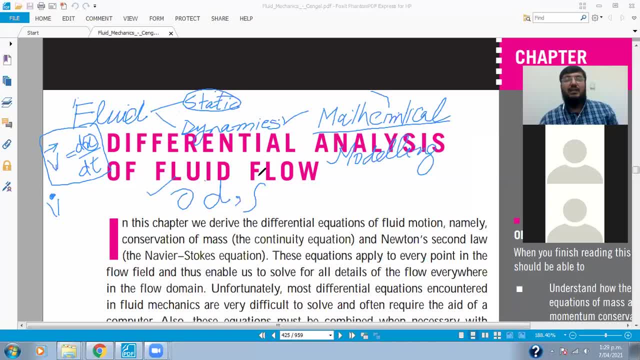 whether it will be a partial or maybe a derivative or integral those three푼 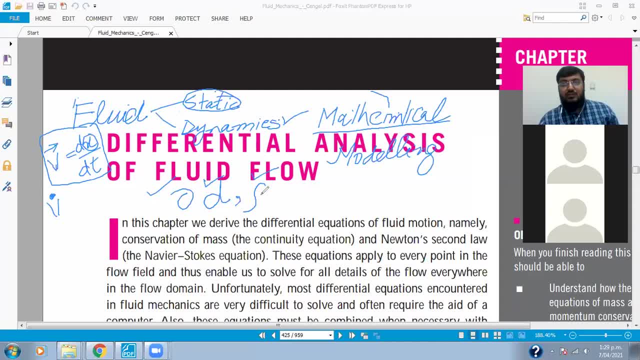 the three are luzarks this is what has been given that are shown 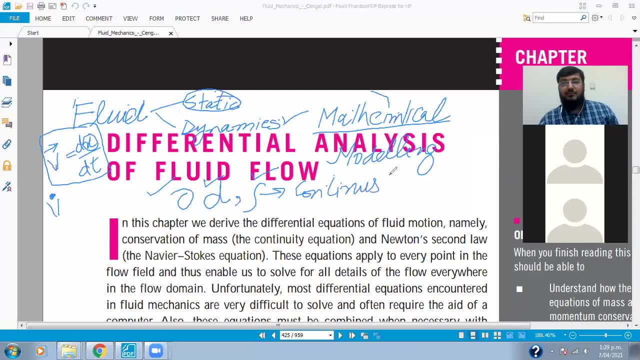 the continuous model ifin years 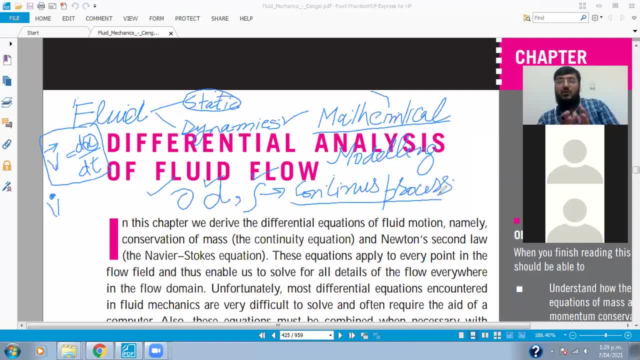 so thatوع will be a key what? so that meio it will be written and how will it be written So it is written, it is short this means that will happen in the form of , it will be written in the form of of know with me, It will be in the shape it will be written. So it will be expressed 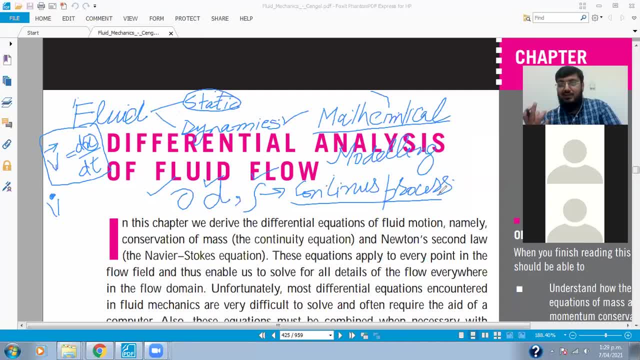 Gan clogui either in the form of partial or in the form of differential or in the form of integral 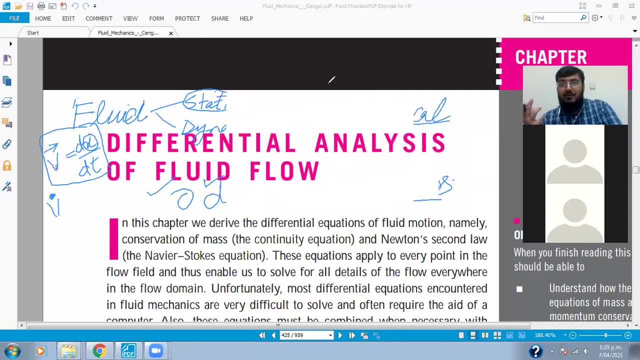 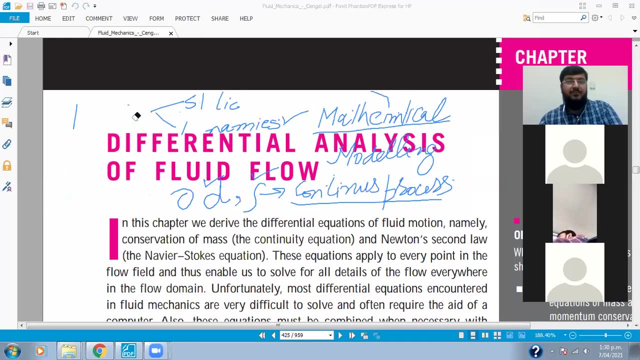 I will tell you later that when to use partial, when to use derivative and when to use integral So we have some mathematical models like this which we have to make Now you see that we have these mathematical models I will raise the score a little mathematical model Now the question is that when fluid mechanics is running So now I say that if fluid is moving from one place to another place 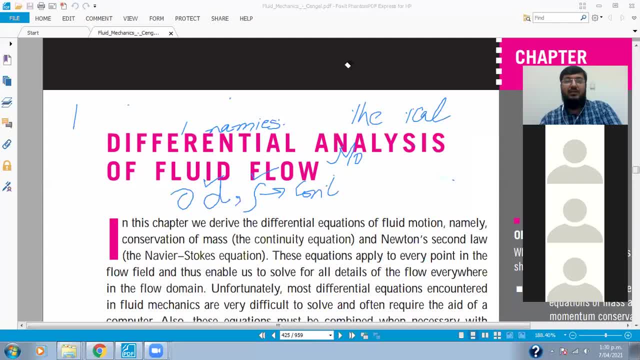 And I have to measure its velocity So I say that okay, you give me its mathematical equation Give mathematical equation or give mathematical model In which I put its value and I get its solution 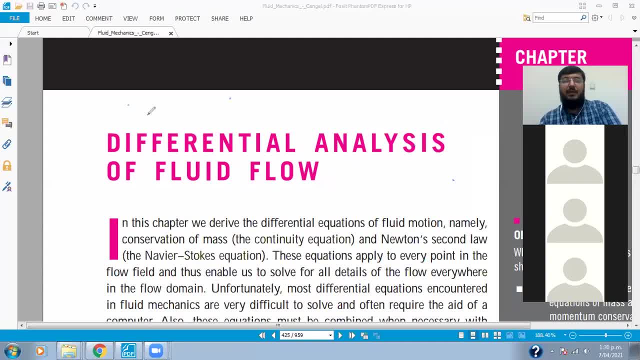 Okay So what will you say? You will say that I mean to say that I need an equation to model the velocity of the fluid 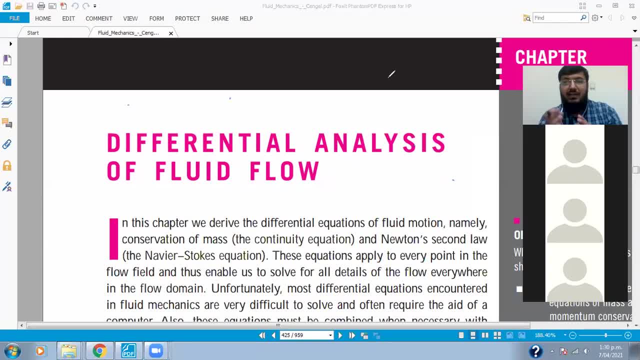 I need an equation to model the velocity of the fluid Now the question is that how will that equation be made? 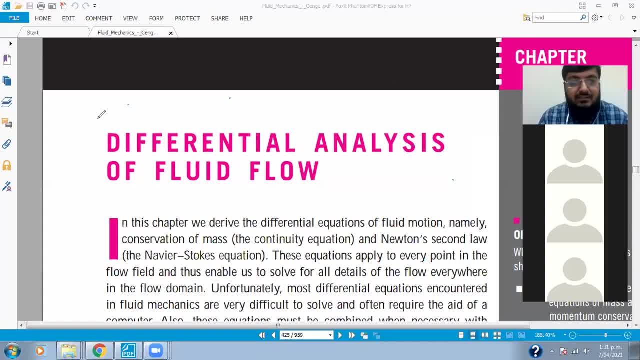 Okay For that son, we have two approaches to do fluid analysis 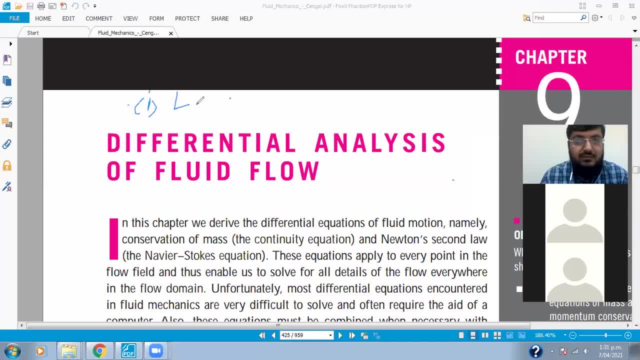 Number one is the Lagrangian approach Let me spend what we gain Number one is the Lagrangian approach Like it is, the standard variable in mysterious 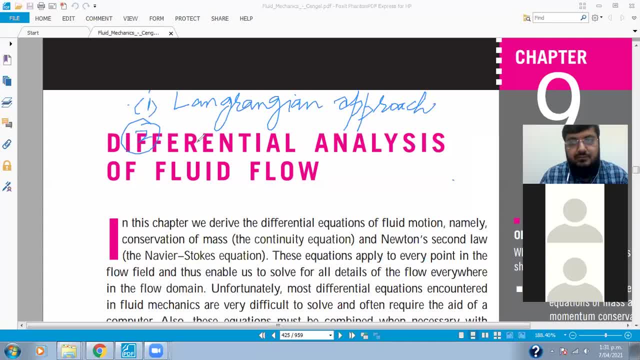 Number one is the Lagrangian approach This is not Lagrangian Number one is the Lagrangian approach 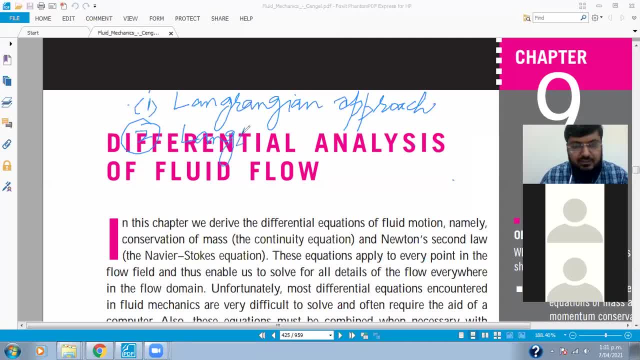 And number two we have I am adding all of them They are being added together 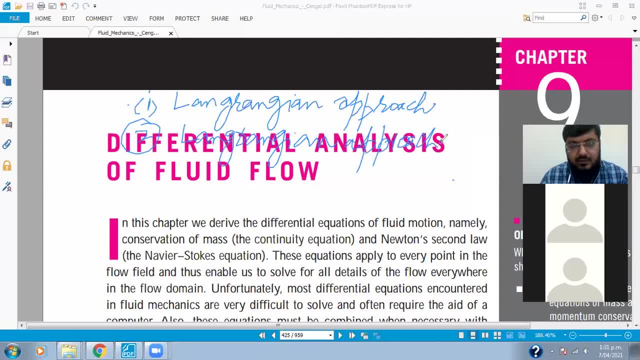 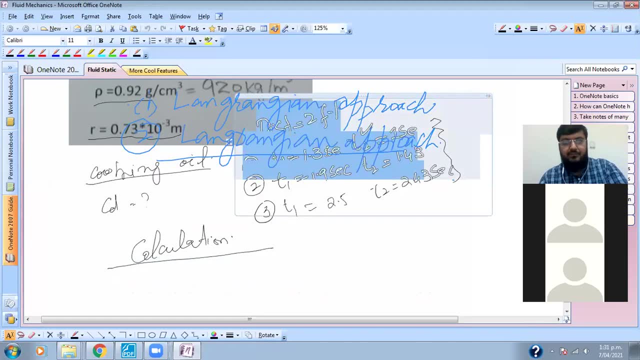 Now, what are the differences between L'engrangian and Eulerian approach, I will tell you a little bit, that why we use this. 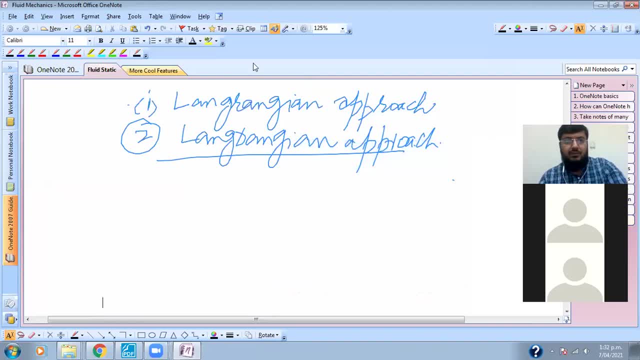 What is the L'engrangian and Eulerian approach we have? L'engrangian approach means that we are... 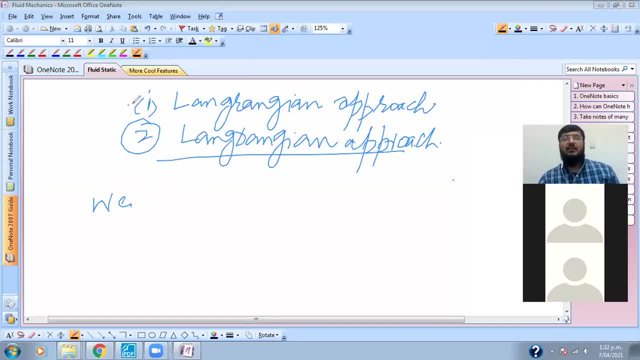 No son, these are two approaches, we will do fluid analysis, this is not the same, L'engrangian and Eulerian approach is not the same. 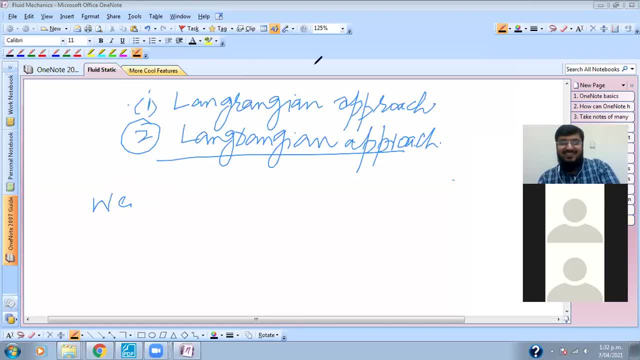 Oh, right, thank you. 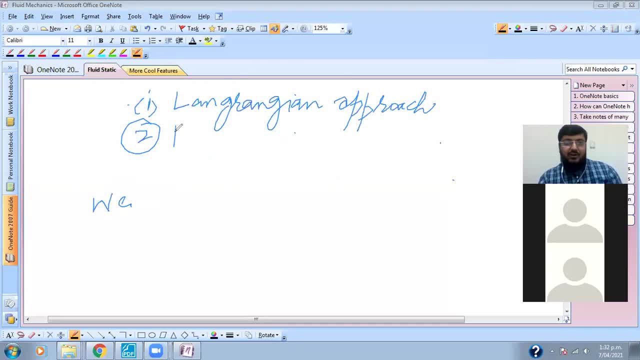 Second, Eulerian approach. Okay. 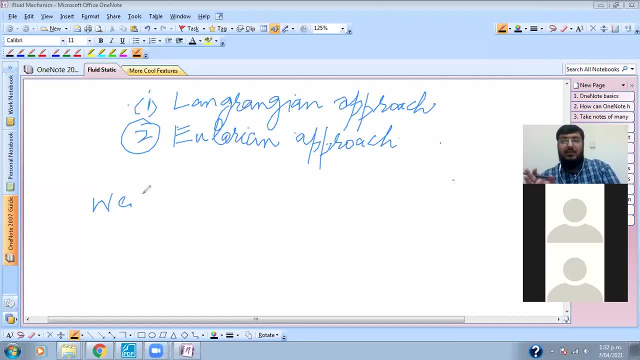 The more important it is to study this subject, the more important it is that the dimension I am taking you to today, you have to understand that story, that why we are studying fluid dynamics too. Okay. So now we have two approaches in it, L'engrangian and Eulerian. 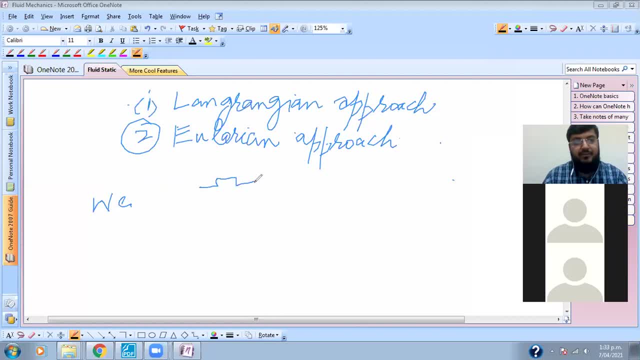 Okay. Now I say that I have a, let's suppose this is a car. Okay. Please understand this carefully. 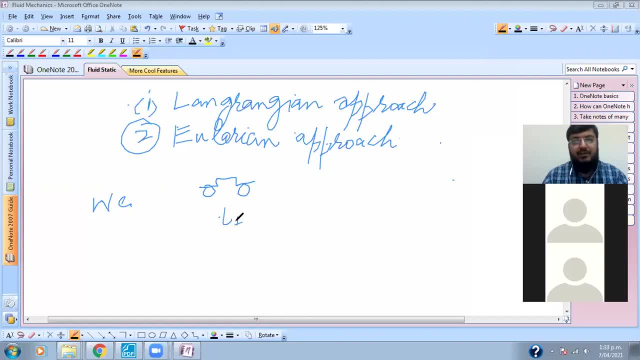 I say that it was on T1 at this position and on T2 at this position. 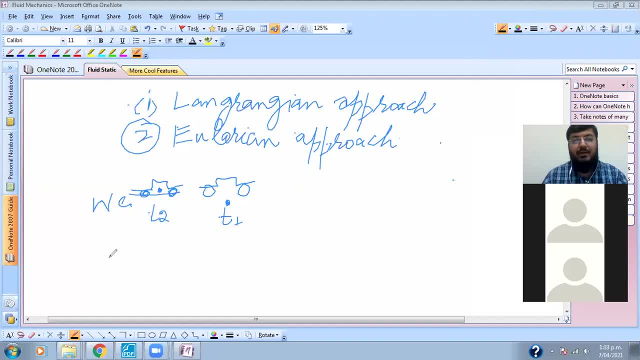 On T2. So now if I have to tell the position of this. So what will I do? 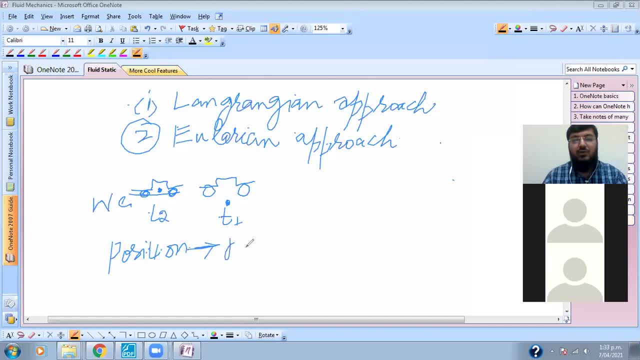 I will say that just, just or only, just single variable would help me. Okay. 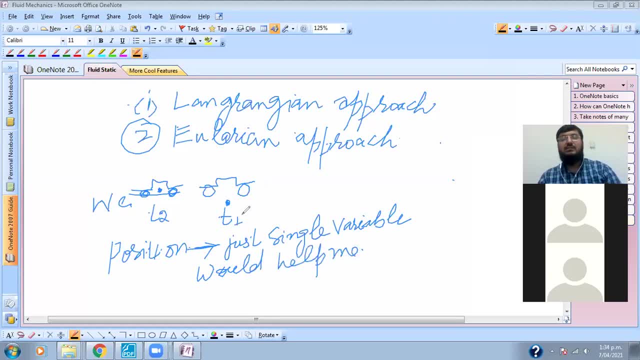 I can tell the position just with respect to time that this car was here on T1 and this car was here on T2. Okay. 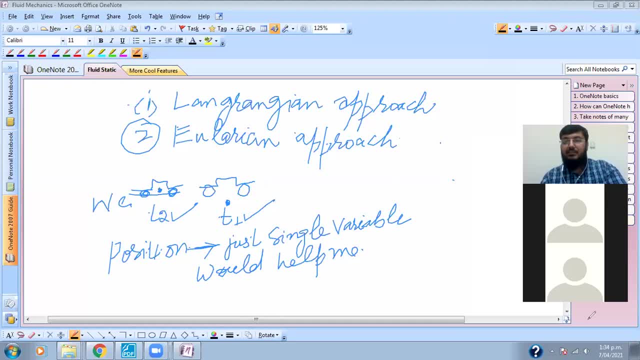 Now if I have to do the same thing for fluid. For fluid. If I have to do the same thing for fluid, then how will I do it? 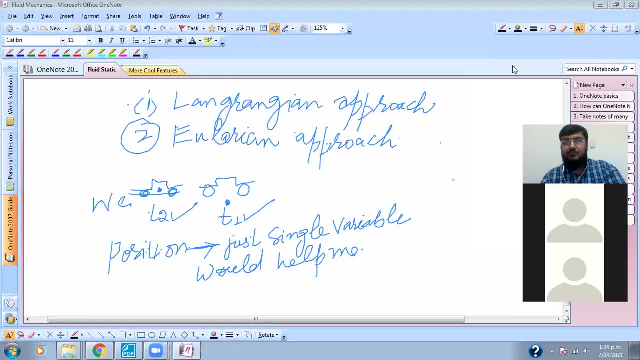 So this is a, I have to do one of these. L'engrangian and Eulerian. Okay. 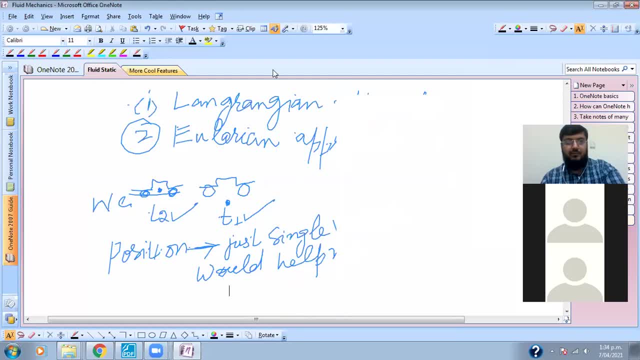 So this is a, I have to do one of these. 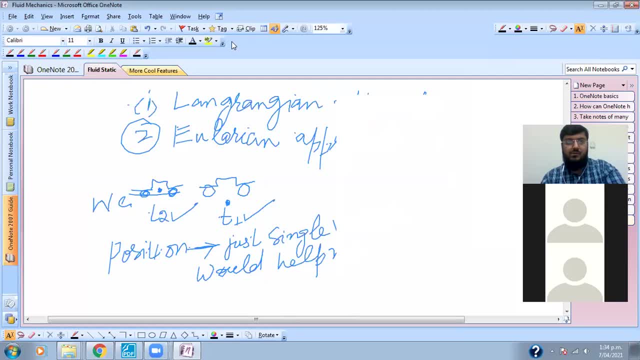 So this is a, I have to do one of these. Okay. So this is a one of these, and this is the one of the two. Okay. 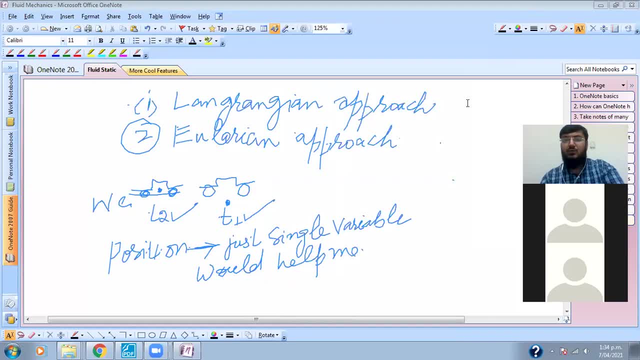 So now I have two more to show you. Okay. So this is one of the two. 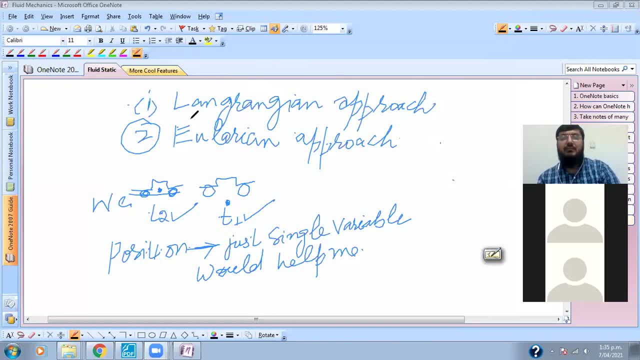 So, the Lagrangian approach is that we have to catch one particle, catch one particle and go after it, catch one particle and go after it, okay. So, this tracing of particle, single particle, this is called the study of single particle, this is called Lagrangian approach. 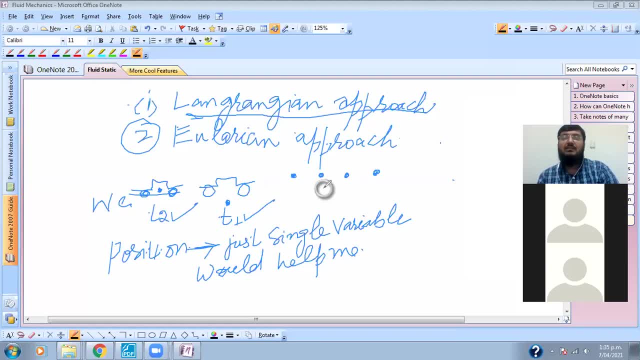 And the mathematical model of Lagrangian approach will always come in the form of D. The mathematical model of Lagrangian approach will always come in the form of D, DX by DT. 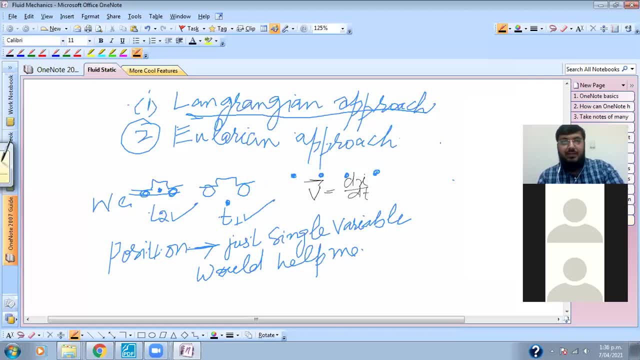 It will come in the form of DX by DT, okay. 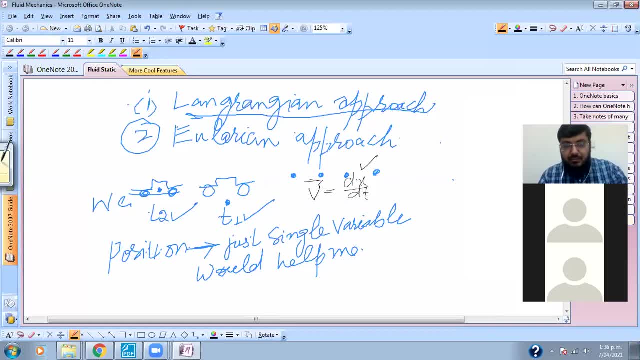 Now, here you see that in the form of DX by DT, if we have any mathematical relation coming, then what does it mean that just single, with respect to X, just in single variable, change is coming with respect to single variable. 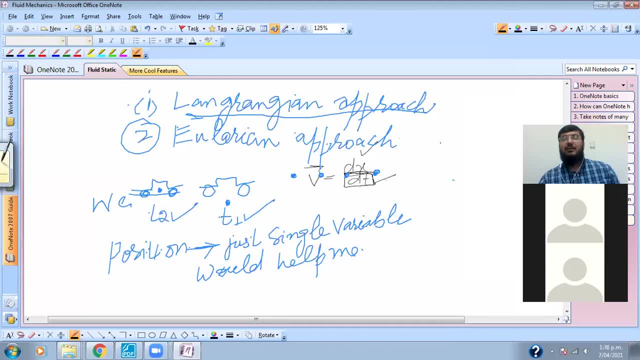 And the one variable we have, independent variable, tells us that the displacement is changing with respect to time. 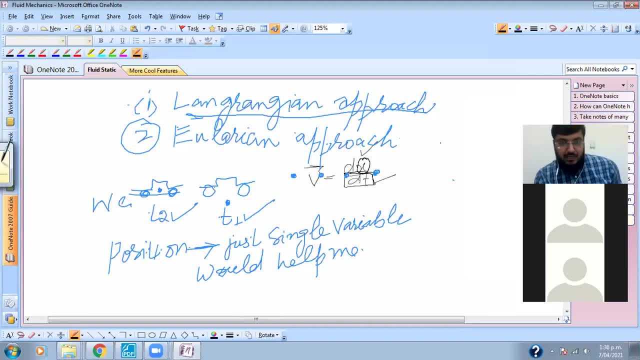 So, the Lagrangian approach means that you start walking behind one particle and start studying it. For example, if I say that if you are going on the motorway, then what is Lagrangian approach, and keep telling that it has reached T1, T2 and T3 so what will be the approach in which the change will come with respect to time that is a Lagrangian approach 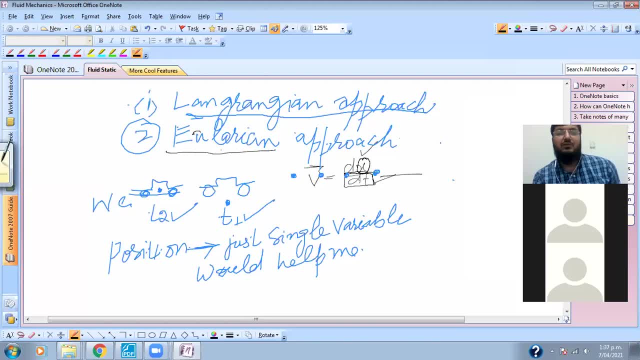 what about fluid, when we talk about fluids then what happens in the fluid is that we can't track a single particle now if a flow is going on in a canal then tell me how the single particle is moving so you would not be able to answer my question, why? the reason is that there are infinite particles in the fluid so for that we have to move on Eulerian approach 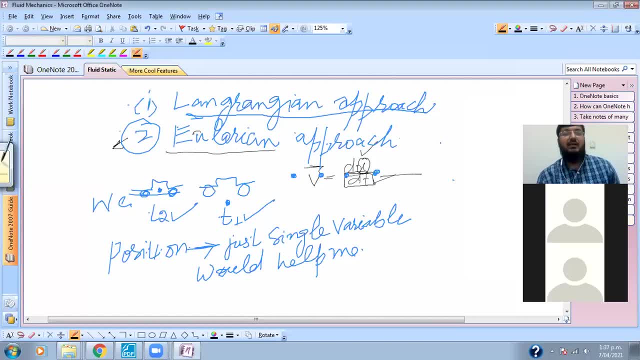 for that we have to move on Eulerian approach what takes us from Lagrangian approach to Eulerian approach we also call Lagrangian approach as control mass system approach what? 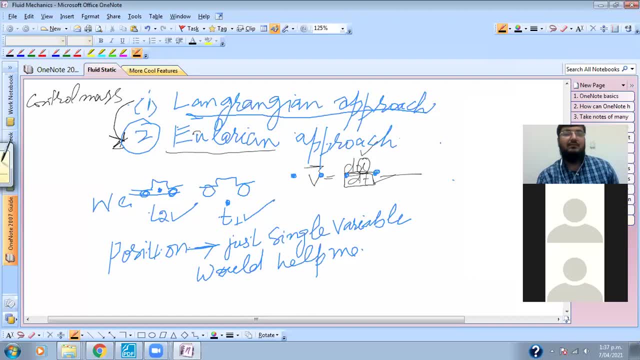 control mass system and Eulerian is also called control volume control volume approach 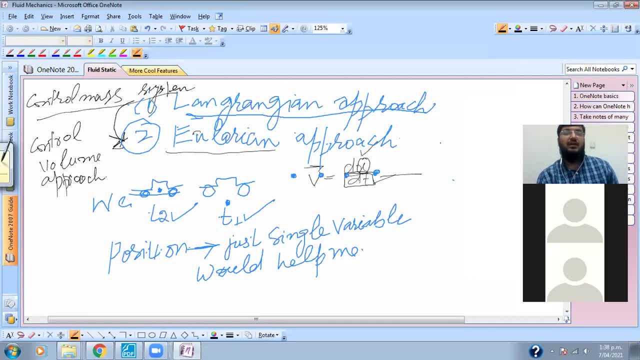 that thing that takes us from control mass to control volume or that thing that takes us from Lagrangian to Eulerian what is the name of that law? can you tell me what is the name of that law? 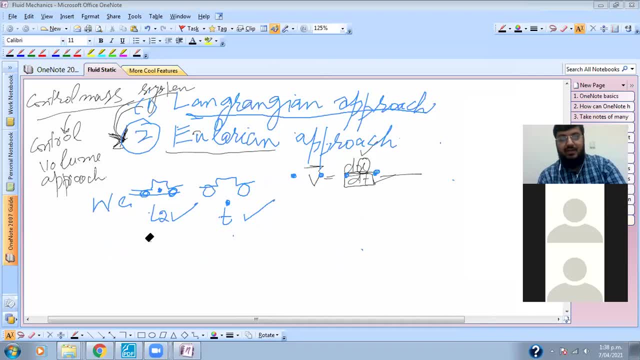 yes son that thing that takes us from Lagrangian to Eulerian or that thing that takes us from Eulerian to Eulerian to Lagrangian that is your that is your yes very good Mobi I don't know who is this Shazi absolutely RTT 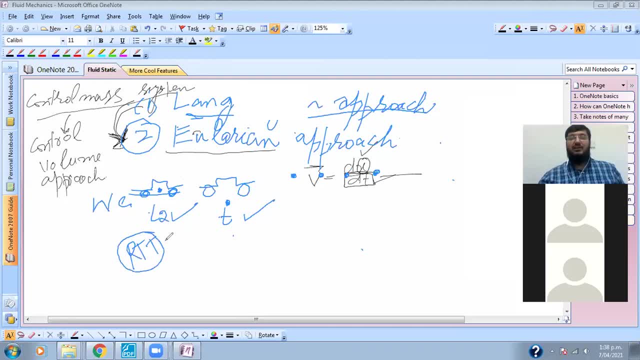 that is Reynald transport theorem Reynald transport theorem absolutely Hammad 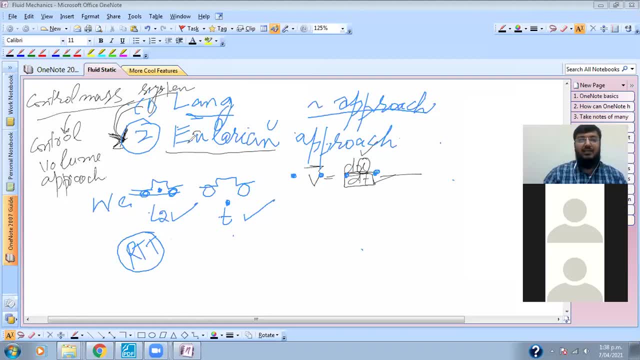 Reynald transport theorem takes you from Lagrangian to Eulerian 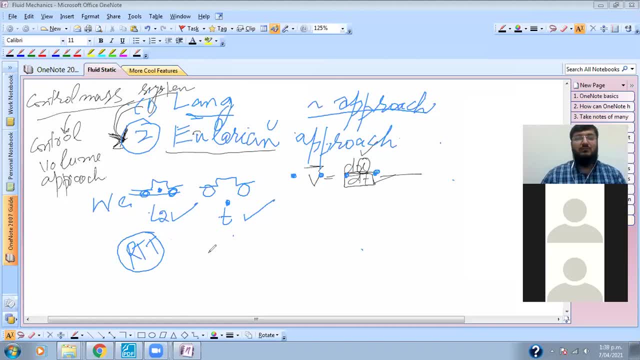 so what is the Lagrangian approach? that approach in which the mathematical models the mathematical equations will come in the form of d dx by dt ok 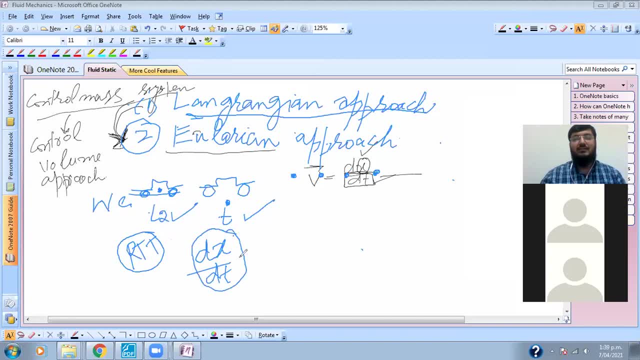 now we have to convert this we have to convert this into integral 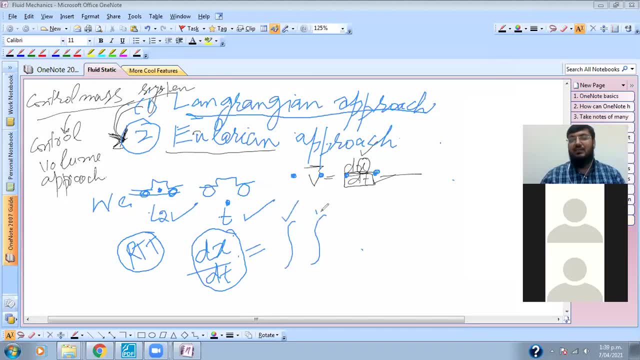 now why integral? the question is why integral? because in Eulerian approach 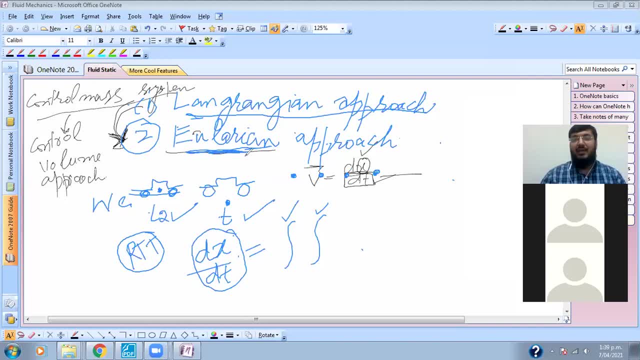 the relation in Eulerian approach will be in the form of integral why will it be in the form of integral? because 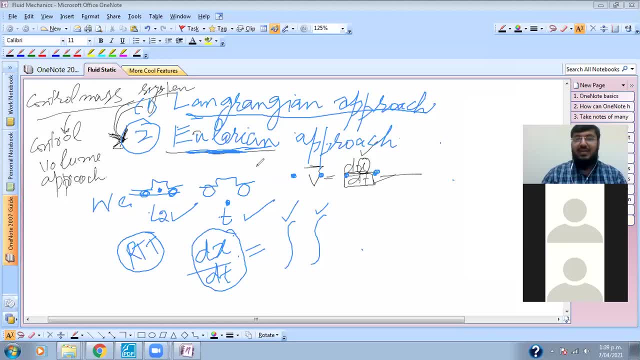 we should know first what is Eulerian approach? 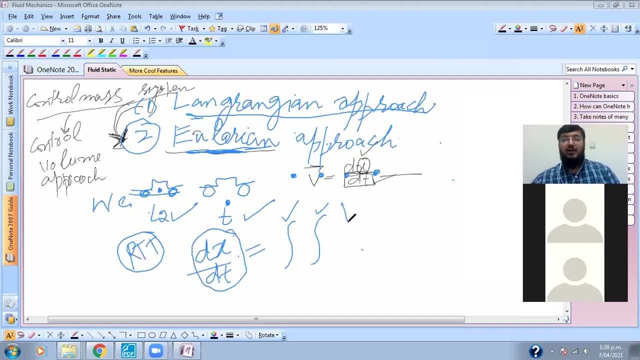 Eulerian approach normally applies to fluids normally applies to what? it applies to fluids why to fluids? because when we take the Eulerian approach because when we take the Eulerian approach it fails 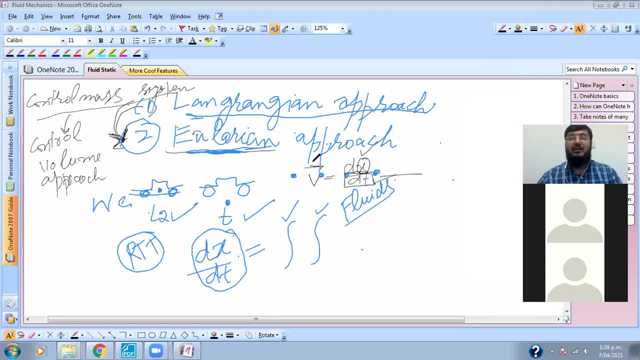 because now we cannot go behind single particles so what do we do? we say that lets do this 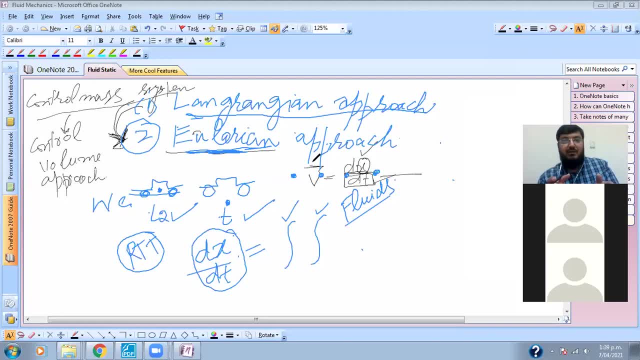 that you place a container at one place for example if I say if I am talking about the canal so we will say suppose you place a small container in the canal in the form of a cube now whatever amount of water is in that container 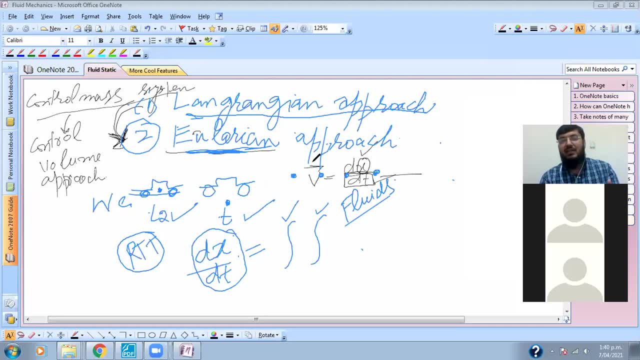 according to the variation of velocity or pressure we will suppose that 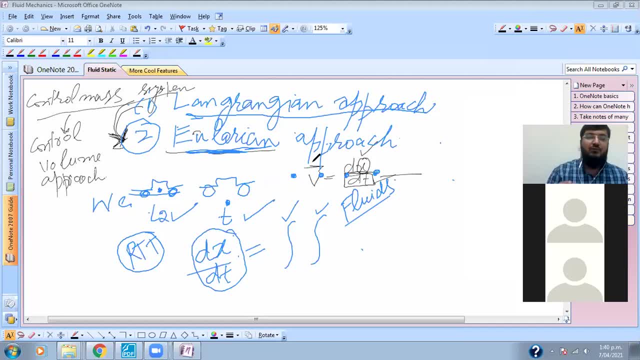 that the velocity of water in the nearby region is the same. The velocity of water in the nearby region is also the same. 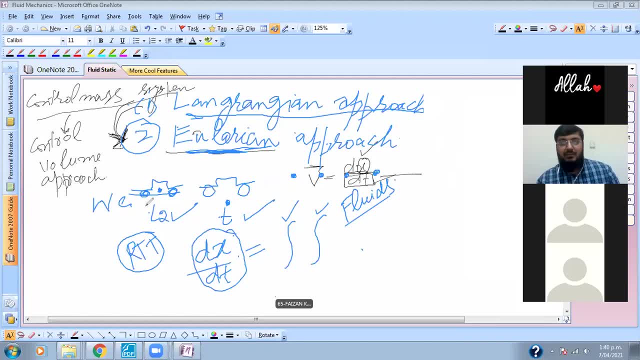 For example, in Eulerian approach, first of all I have to suppose a control volume. What do I have to suppose? Control volume. I have to suppose a control volume. I have to suppose a container like this. I have to suppose a container in the form of a rectangular form. And I suppose that the way the water will behave in this container, it will behave in the same way in that canal. 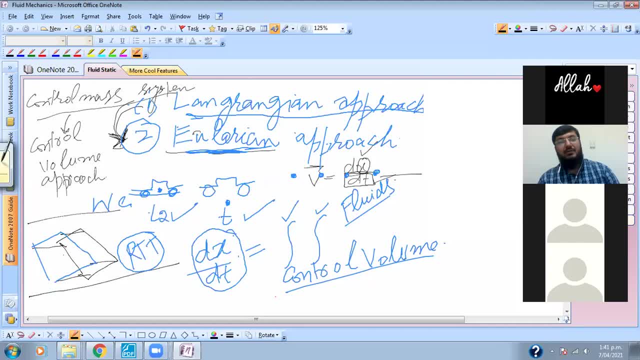 Now if this control volume, now if this is the control volume, now the variations that will come in this control volume, we have to measure them. 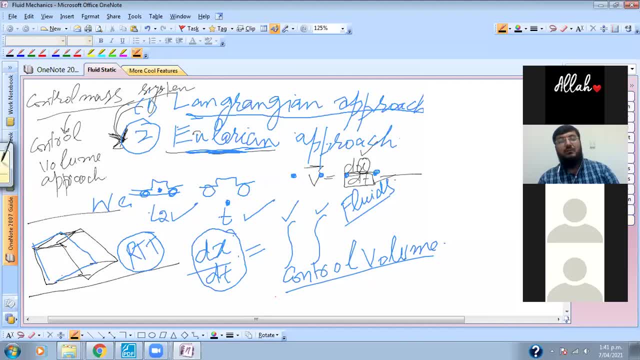 Now if I see this container, there are two things in this container. One is its boundaries. That means if I talk about a glass, if I talk about a container, let's suppose if this is my mobile. Okay. 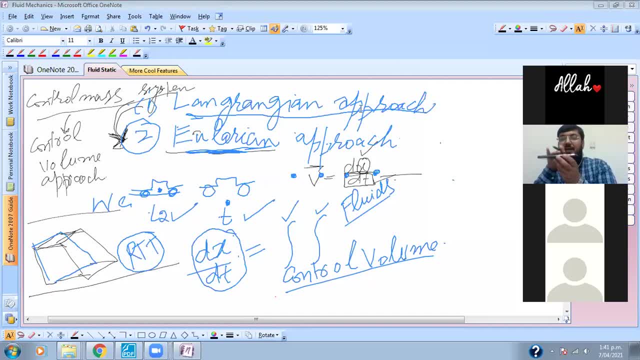 If this is my mobile, then one of the surfaces of this mobile, the surfaces of the container are the boundaries. Boundaries are normally called space. 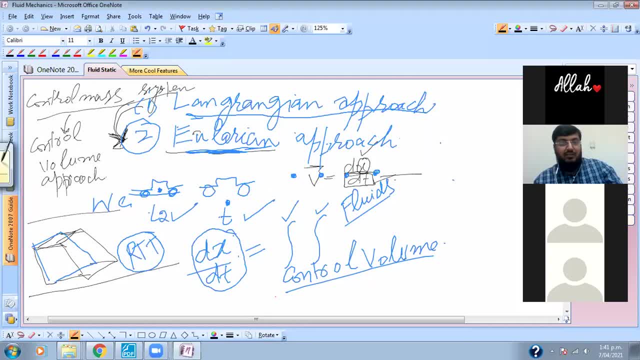 That means if I have to move the boundary in X axis, this one is its X axis, this one is its Y axis, and this one is its Z axis. Okay. 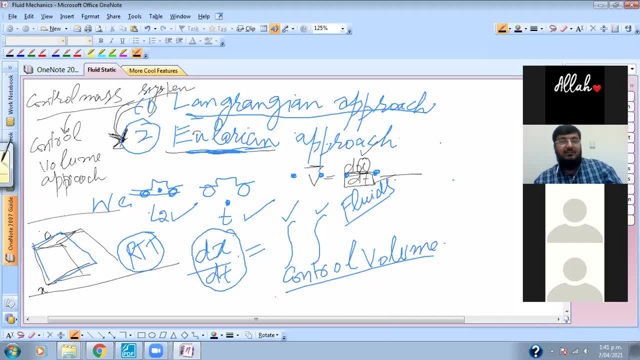 This one is X axis, this one is Y axis, and this one is Z axis. 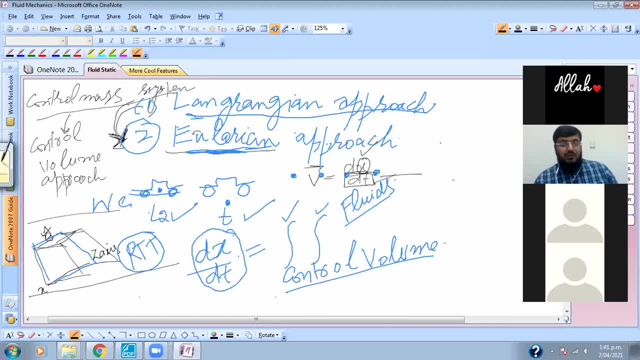 Okay. Now if I have to move normally in boundaries, in which I have to move? In boundaries. So how do I have to move? How do I have to move? I have to move. Exactly. Exactly. Exactly. 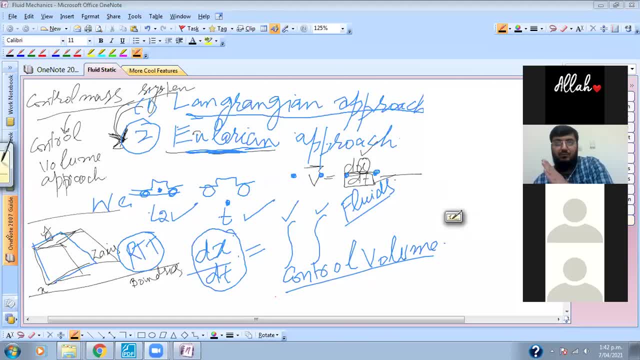 Son, you know, if you suppose that we are talking about pipeline, then it will mean that you are considering your control volume in the form of pipe. 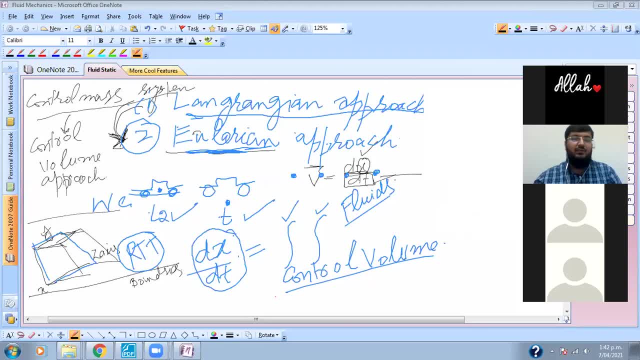 Now because I have kept this cuboid, it means that I am considering my control volume in the form of a container. Okay. So you can take control volume of any shape. Okay. 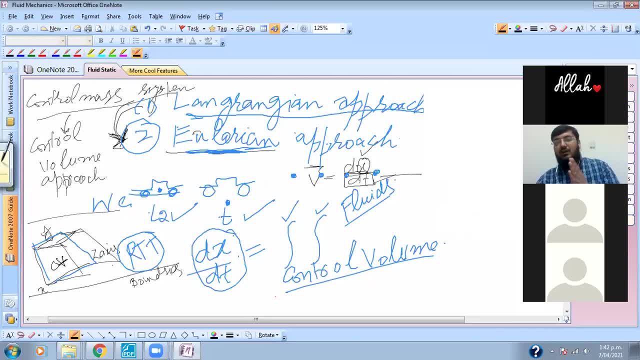 So normally what is taken is taken as cuboid for understanding, because its Cartesian coordinate comes in it easily. Okay. 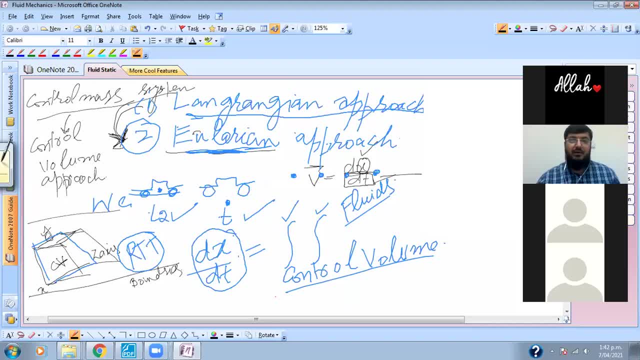 So now when I talk about control volume, there are three things in it. One is its axis, XYZ. So this means that when, if we talk about control volume, then the change in it will also come with respect to space. Space means XYZ. If I talk about this container, okay, if I talk about this container, then in the container, suppose if I draw a picture in one time instant, that is, what we did not play in childhood, that the next person used to say stop, then it used to stop there only. 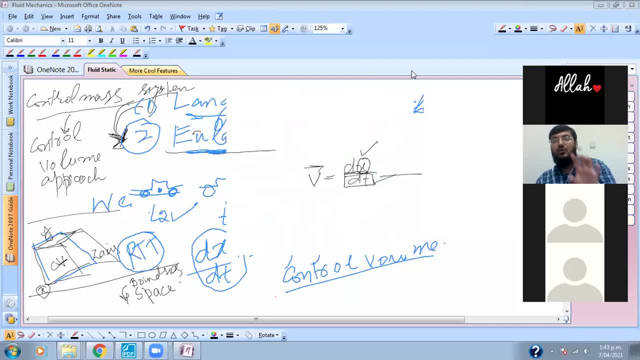 So similarly, you have to suppose that if I stop the fluid in that control volume, then if I say that in that rectangular shape of mine, let's suppose if this is my container, then in it, this is the axis, this is the X axis, this is the Y axis, and into the page, this is the Z axis. 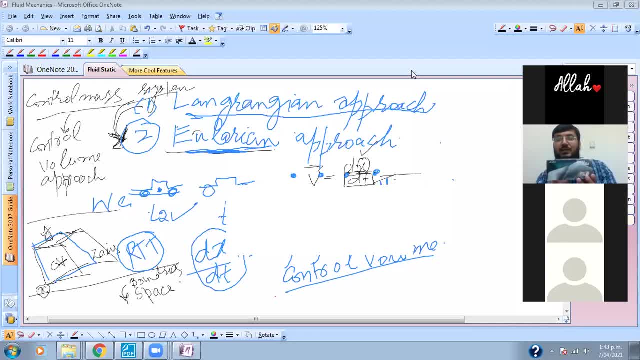 So if I say that, okay, you find its velocity on every particle of it, then this is our imagination. Definitely, 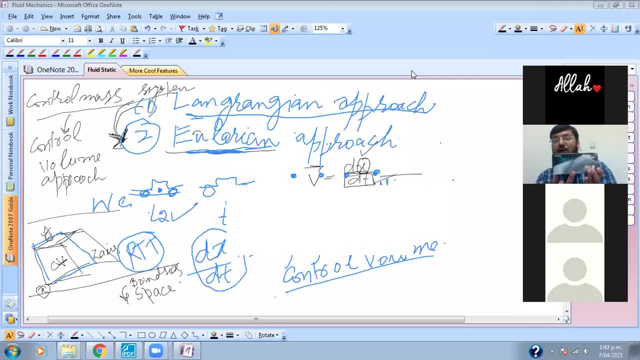 the velocity in the X direction, it will be different at every point. Its variation will also come along the X velocity, and it will also come in Y, and it will also come in Z. Okay. In a container, 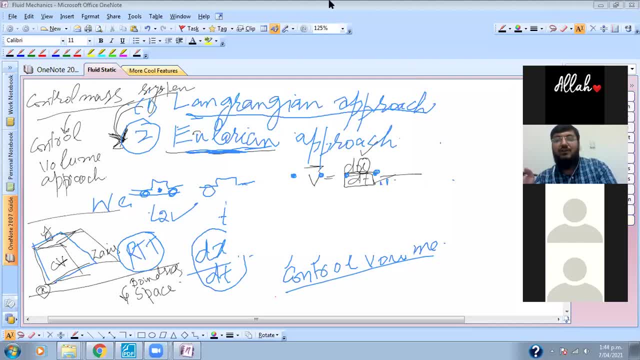 the velocity on every dimension will be different. Okay. 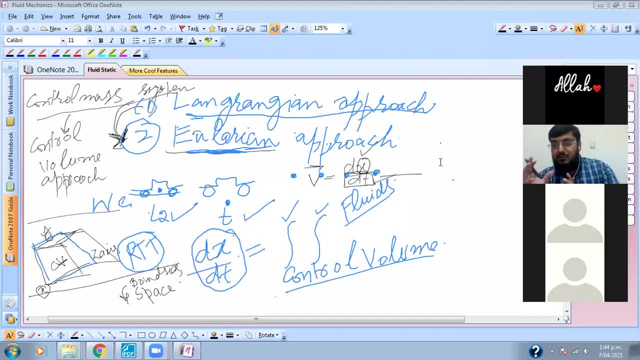 So this means that when we talk about Eulerian approach, then we are supposing a control volume. Now, the change that will come in the control volume, 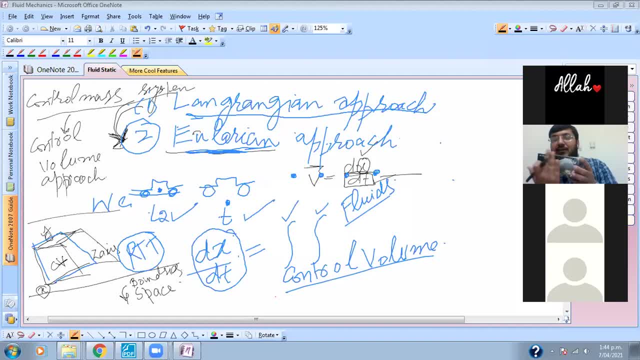 And with respect to time, if I say that in T1, this container was completely filled with water. 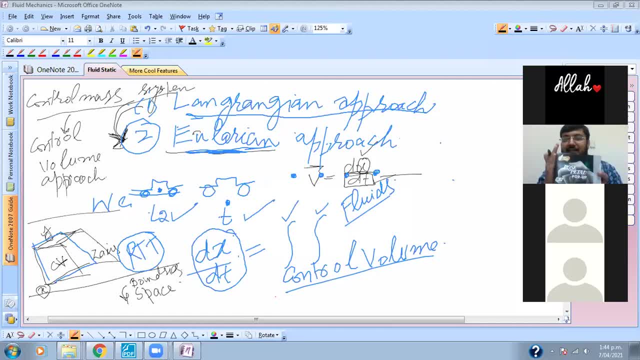 Now, if new water came in T2, then the old water, obviously, it has gone ahead. So the new water that has come, it will have a net velocity again. Suppose, water has entered in it first at 2 meters per second. Now, if new water has come, then it has entered at 3 meters. So now in this control volume, 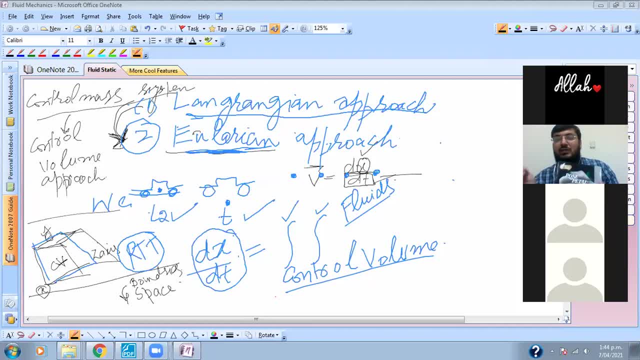 with respect to time, the change is also coming, and with respect to space, the change is also coming. 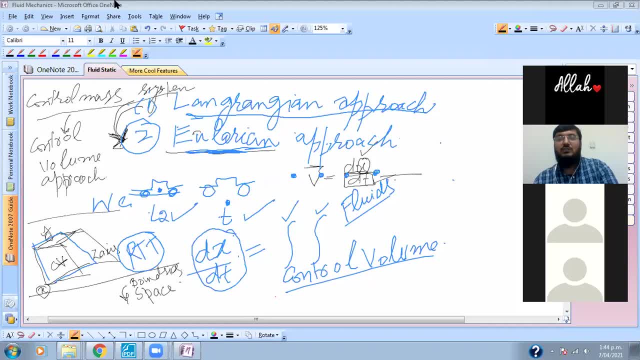 It took time, with respect to time, the change is also coming, and with respect to space, the change is also coming. Okay. 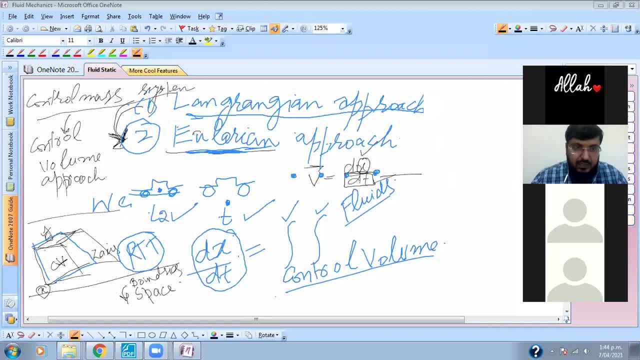 So the Eulerian approach that we have, the Eulerian approach that we have, in that, with respect to space, the change that comes with respect to space, that would be time. 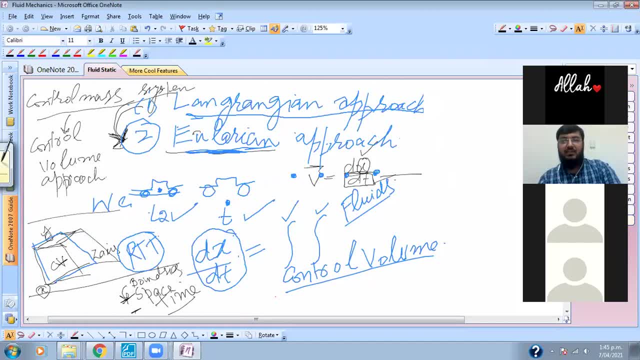 Time and space, both of them, both of them, our change will come. 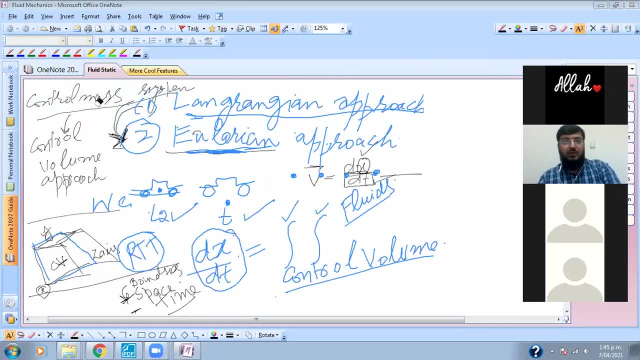 So now, if I raise all these things, I will tell you an easy way to tell you about it. The method is, give me some time, it takes some time. 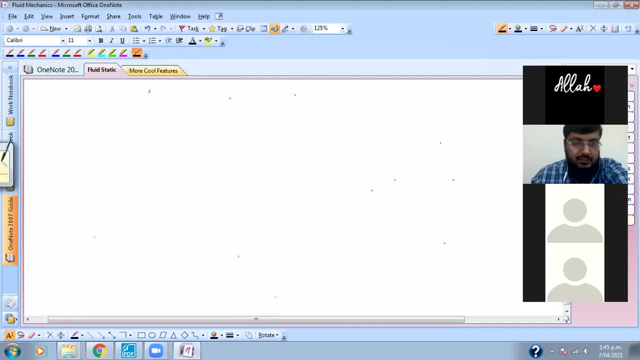 Okay. Now let's start, that we have two approaches. Okay. 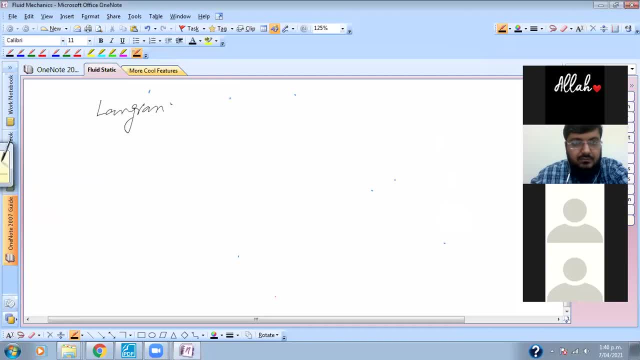 One is Langerangian. And the second approach is Eulerian. 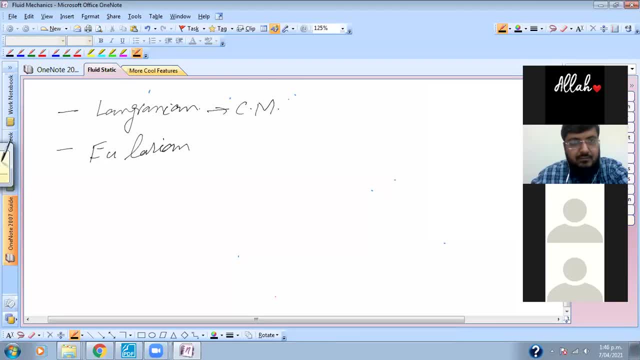 This is control mass system, and this is control volume system. Okay. This is control mass, and this is control volume. Okay. 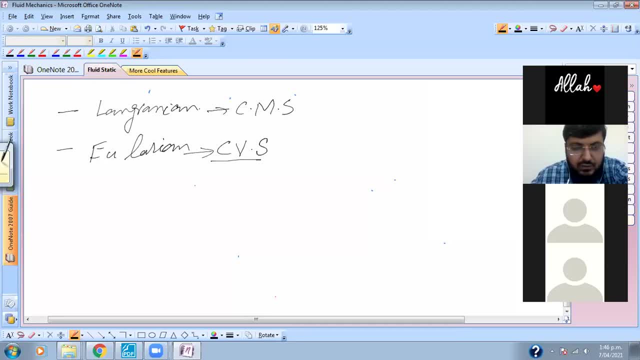 Now, the control volume approach that we have, the change that will come in this, with respect to time, plus space. 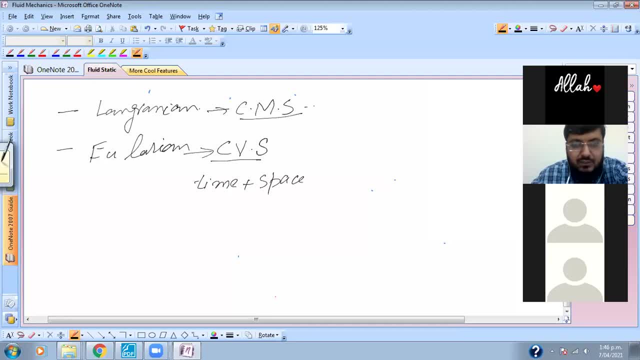 And the control mass system, the change that will come in this, with respect to single variable. 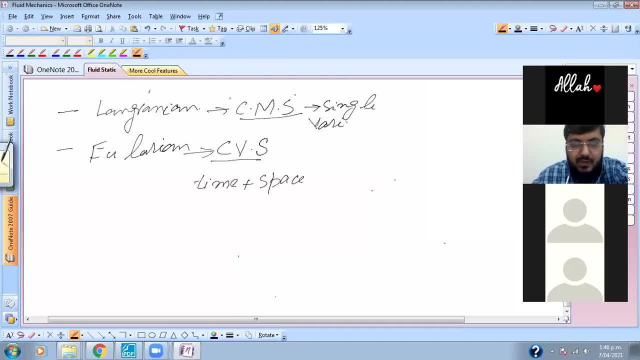 That is, it can be time, it can be space. These two approaches, you have to understand that, the Langerangian approach is that, 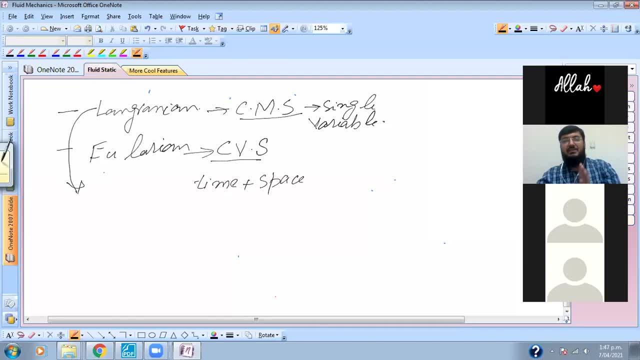 you are standing on the motorway, if you have to follow a car on the motorway, then you have put a car behind it. 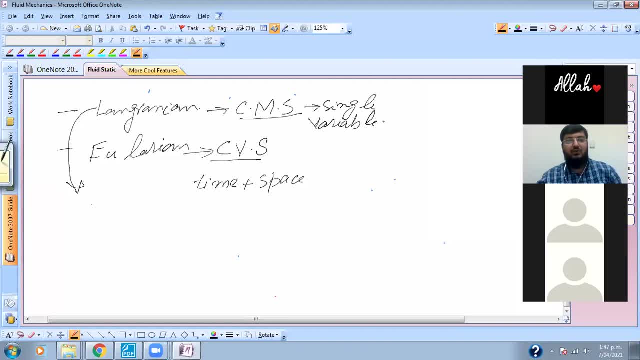 So, that will be the Langerangian approach, the change that will come in it, with respect to that, when its mathematical model will be made, then it will be in the form of dx by dt. The Eulerian approach will be like this, that partial v by partial t, time, plus, partial v by partial x, plus, partial v by partial y, plus, partial v by partial z. So, this is what you have, 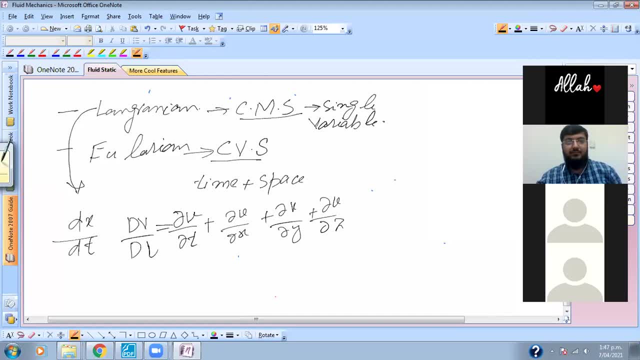 dv by dt. Okay? Now, the Eulerian, 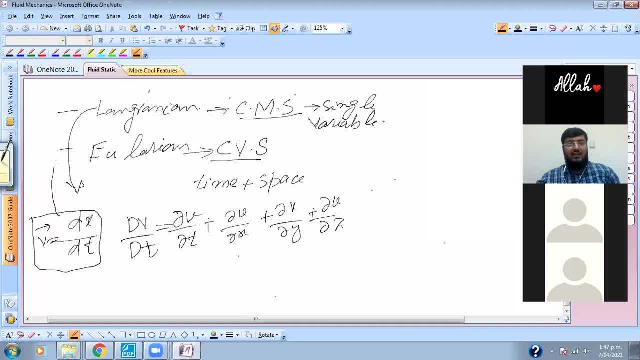 the Langerangian approach, the relation will be like this. 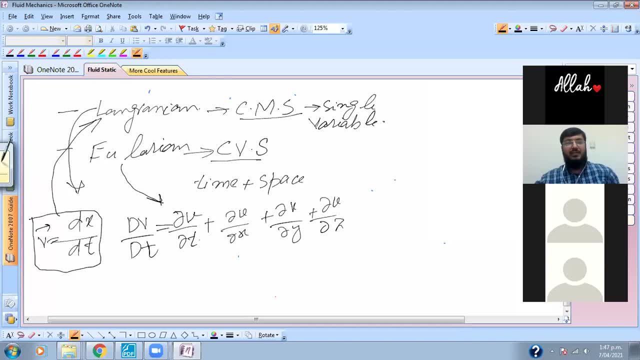 The relation of the Eulerian approach, will be like this, which will tell us that, 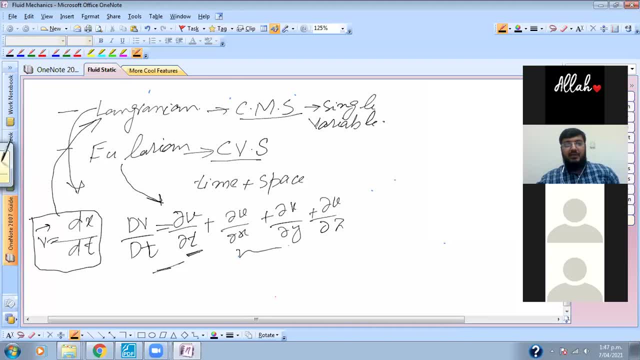 if in any variable, with respect to time, plus space, with respect to time, 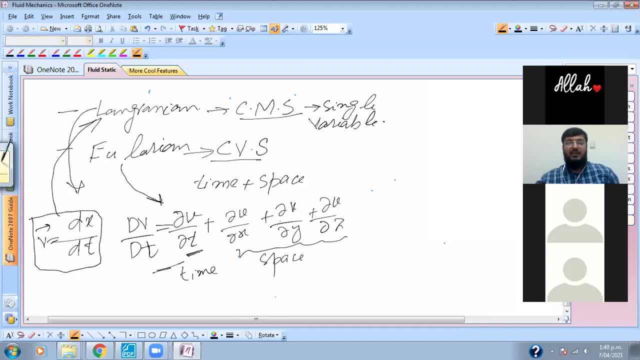 plus space, there is a variation in both, then we will have, I will repeat it, one minute, Kasim, I will repeat it. 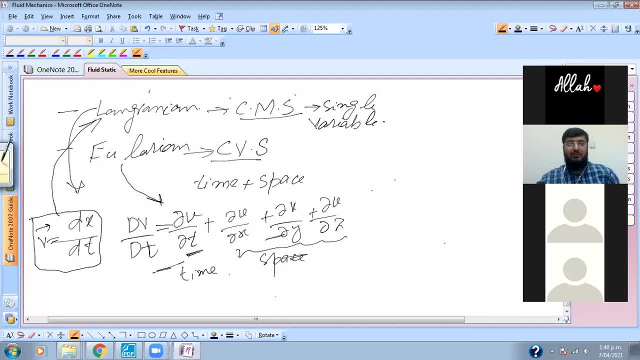 If we have time, plus, time, plus space, there is a variation in both, then what will we have? 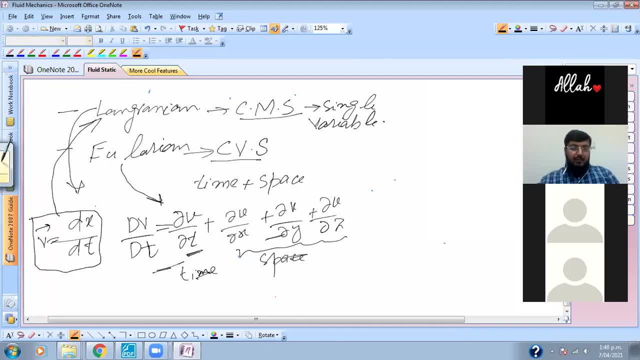 We will have the Eulerian approach, and if we have only one derivation, 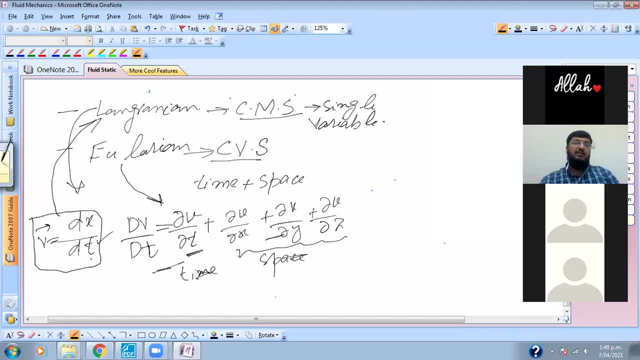 a change in a single variable, then we will have, what will happen? 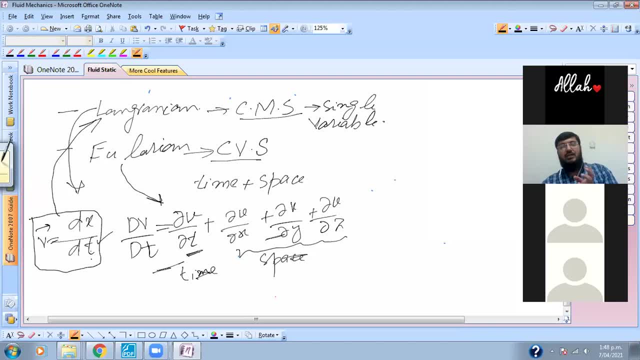 The Langerangian approach will happen. I mean, the Langerangian approach, you have to suppose that, there is a motorway, you have put a car on the motorway, you go behind the car, then how can you define the position of the car? Just with respect to single variable. You will say that, it is here on t1, it is here on t2, or you will do it simply, that the plane is going, 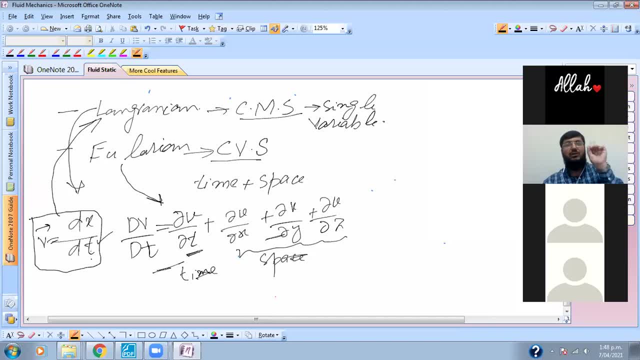 if you want to follow the plane, then you can easily tell the plane, that it was here on t1, it was here on t2, it was here on t3. Okay? 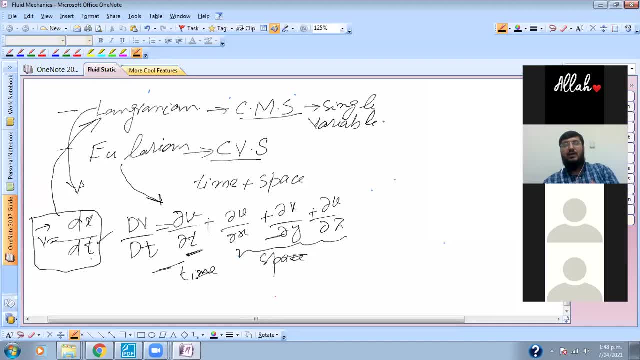 With respect to single variable, if there is a change in it, then it is Langerangian approach. It is Langerangian approach. 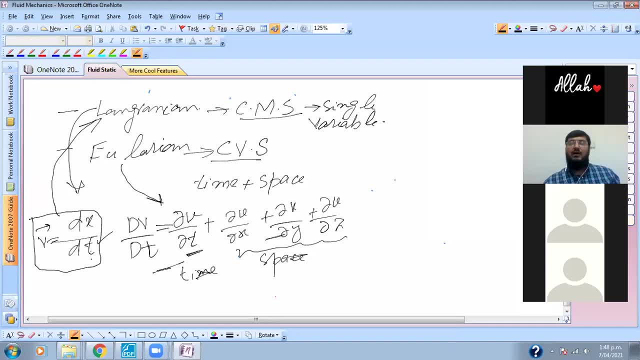 The meaning of Eulerian is, that you are standing on the motorway, you cannot follow every car, if the number of cars is more. 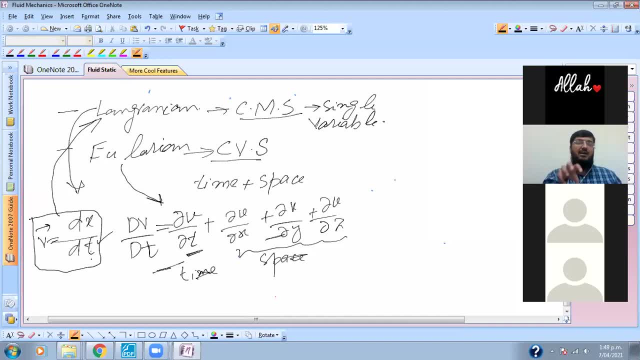 So, what you do is, standing on the motorway, you have put a camera. You say that, I am not concerned with this thing, 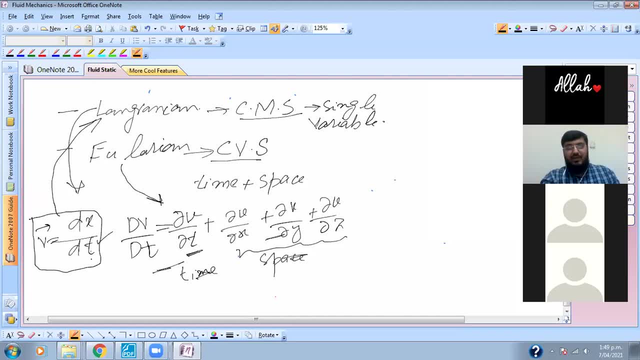 that the cars in the vicinity, how they are behaving. You have to say that, the way the cars will behave in my radar, 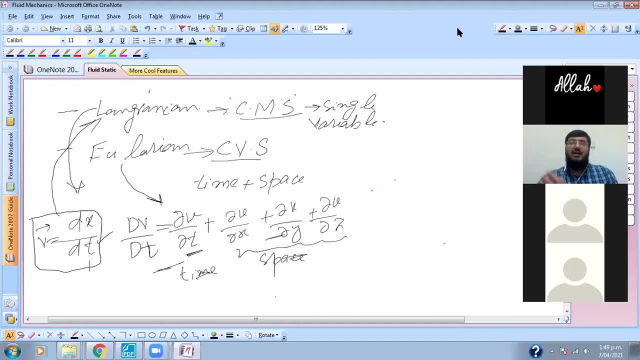 I will suppose that, there are other cars on the motorway, how they are behaving. 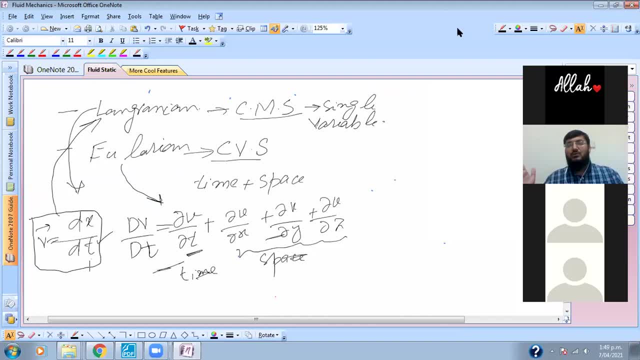 So, you have put a camera on the motorway, whatever car passed through that camera, the velocity of that car, you have to suppose that, it is coming from behind with the same velocity. 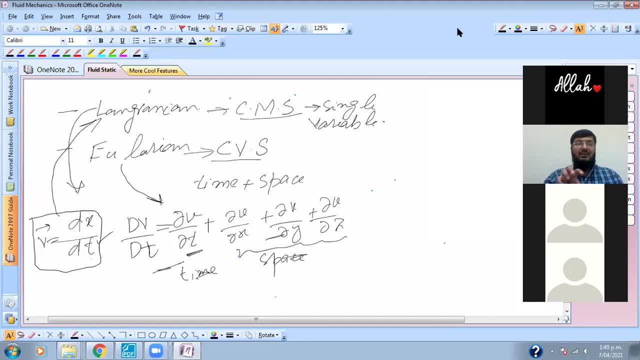 This means, it will happen that, it is coming with the same velocity in the camera. Okay? 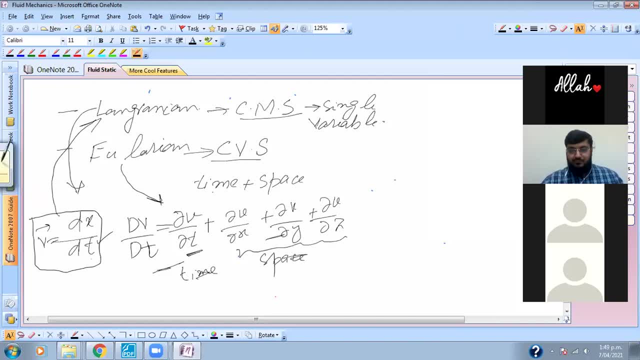 So, now it will happen that, now you see that, let's suppose, if I say that, if you are talking about the camera, if you are talking about the camera, then suppose the radar was this much. Okay? 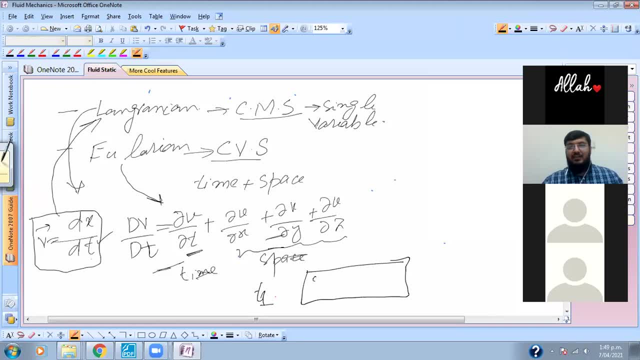 So, let's say, over T1, if here, here, here, here, here, here, this car came, suppose, if over T1, 10 cars have come, Okay? Then when T2 goes, then it may happen that, 12 cars may come in this radar. And this space, which 2 particles, 2 cars which was in this position, it may happen that, at the next time instance, some new cars will come here. 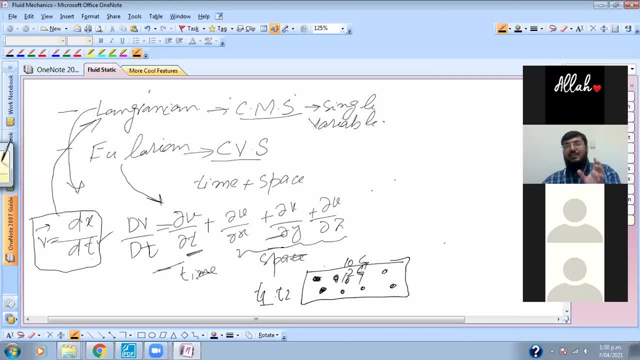 So, an eulerian approach in which you have fixed a box, you have fixed your control volume, volume fix kiya hua hai, ya apne apna analysis karne wali jo apki domain hai, wo apne fix ki hui hai, wo apne fix ki hui hai, wo apne fix ki hui hai, to usko, wo jo apne fix ki 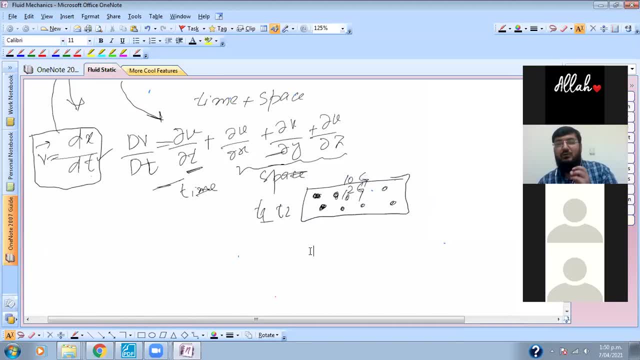 hui hai, aap usme dekh rahe ho ke aapki jo changes hai, with respect to time plus space dono me aari hai, that is called Eulerian approach. 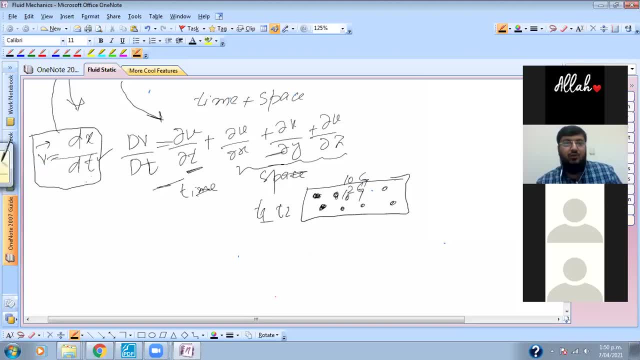 Aur Lagrangian me kya hai, ke jab uska mathematical model banega, to wo just with respect to single variable ki form me banega, wo with respect to single variable ki form me banega, theek hai, I hope ki ab aapko Lagrangian aur Eulerian ki bilkul samay lag gayi hogi, ke agar kusi relation aisa hai, jisme with respect to single variable hai, theek hai, to wo kon sa hoga, wo Lagrangian approach hoga, aur koi aisa relation jisme time plus space dono aare hai, to wo kon si approach hogi, wo Eulerian approach hogi, lekin mera yahan pe ek chota sa question hai, aap logon ke liye, theek hai, question mujhe answer kare, aap 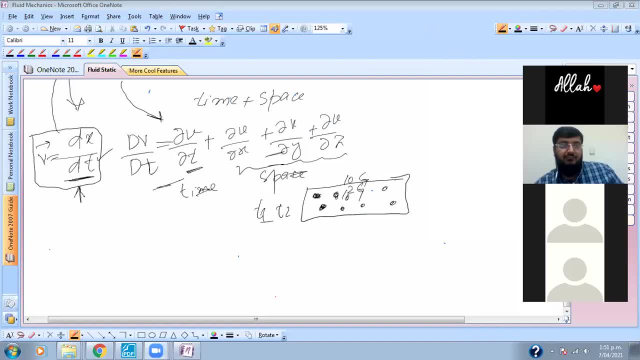 log, ke aap logon ke liye, jab maine V vector likha yahan pe, to maine iske saad chota D laga diya, 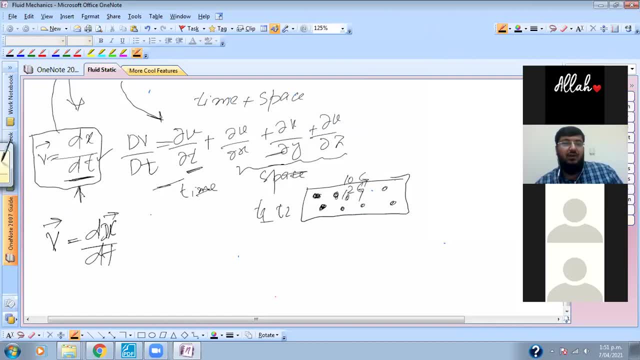 kya laga diya, chota D laga diya, theek hai, aur jab maine ye Eulerian approach ka likhi relation, to yahan pe maine partial laga diya, to ye mujhe pata kaise chala, maine isko aise nahi likh sakta tha partial x by partial t, V is equal to, kaise nahi likh sakta tha 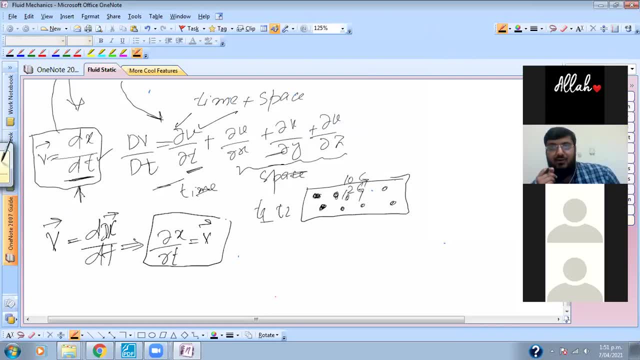 maine isko, maine isko sa derivative kyu laga ya,